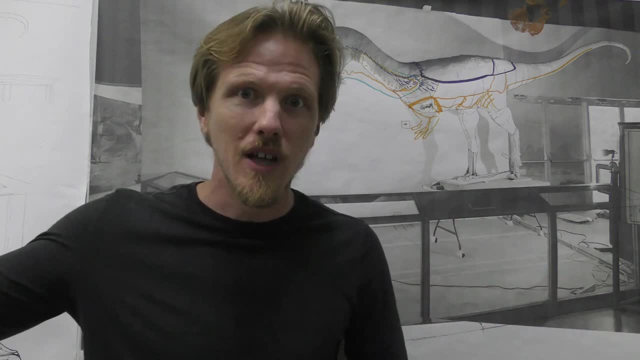 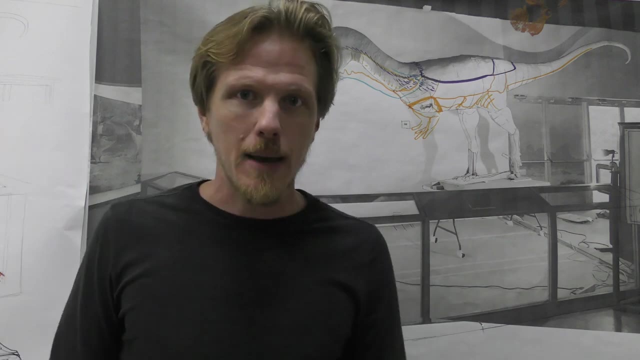 holds a record of what was going on with the Earth's CO2 levels in the atmosphere and dissolved into the ocean. We have a record of the Earth's climate and how life is adapted to it, in the geology of our planet And as we move into the 21st. 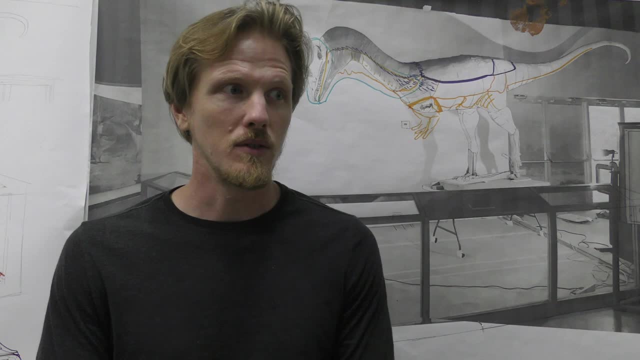 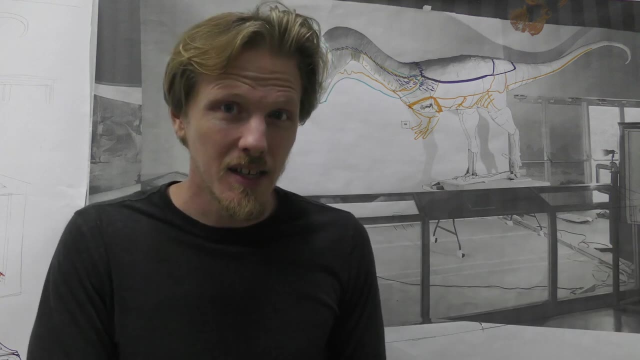 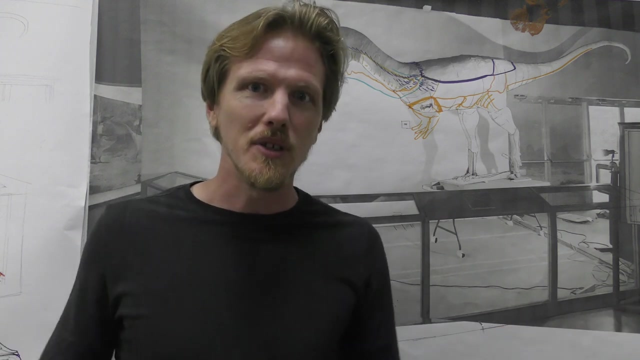 century. we're getting hit daily by crazy events related to human induced climate change, Climate change that was predicted all the way back in the 1960s, The evidence for which was pretty unequivocal in the 70s. and here we are, 50 years later, basically completely unprepared. 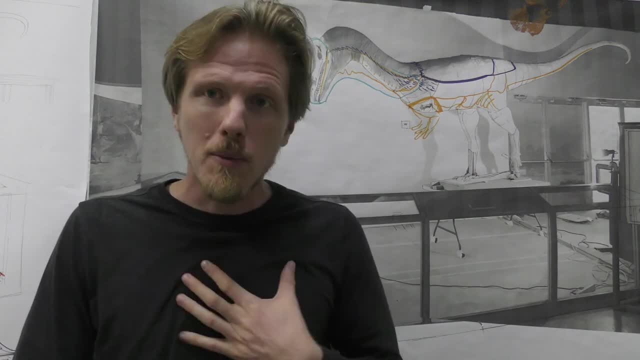 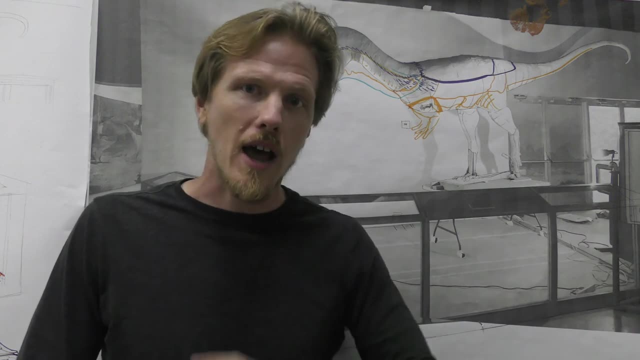 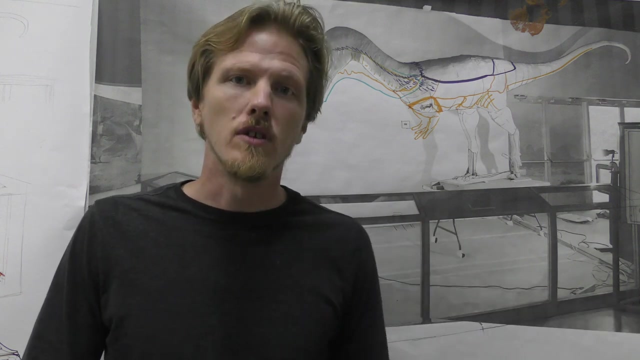 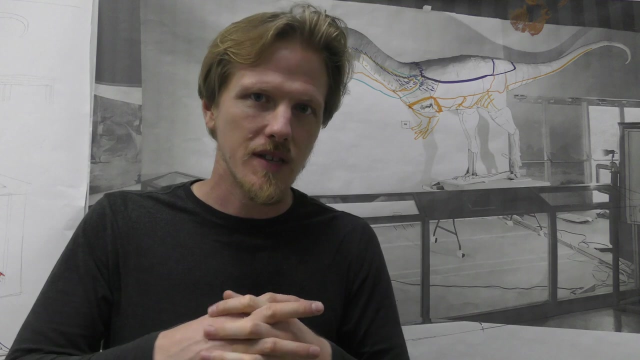 you. So, from my perspective, it seems like the only thing left to do is to try and educate the entire public about how our planet works, so that the voting public can make good decisions about what they vote for and what they pay for. moving forward, Paleo art synthesizes a vast amount of scientific data from the 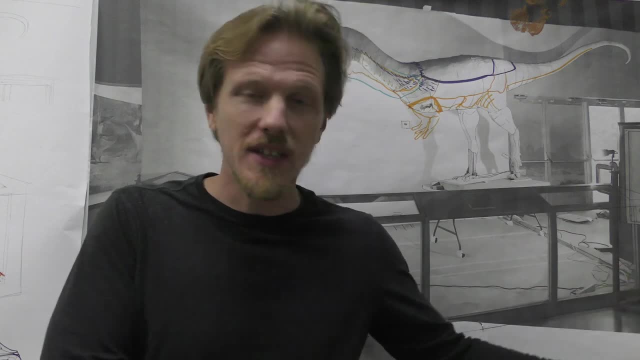 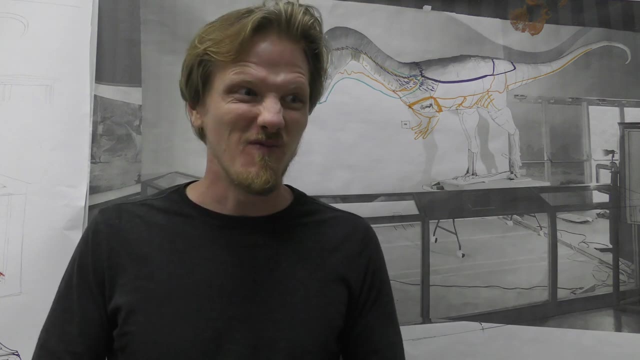 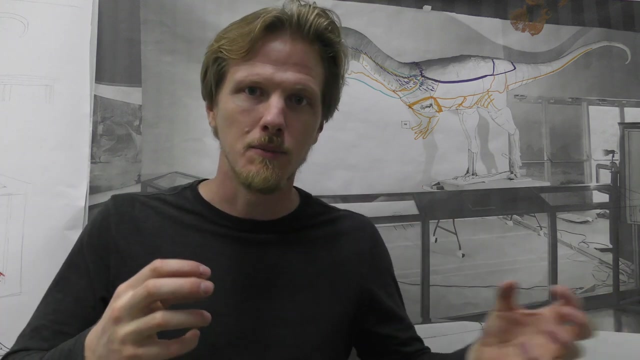 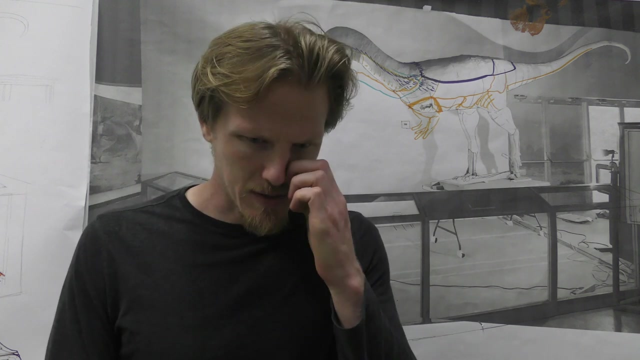 fields of science that allowed people to predict that stuff back in the 60s, that allowed people to predict the disasters we're going through over 50 years ago. Paleo artists are an important link between the academic scientific community and the general public, So as the Society of Vertebrate Paleontology. 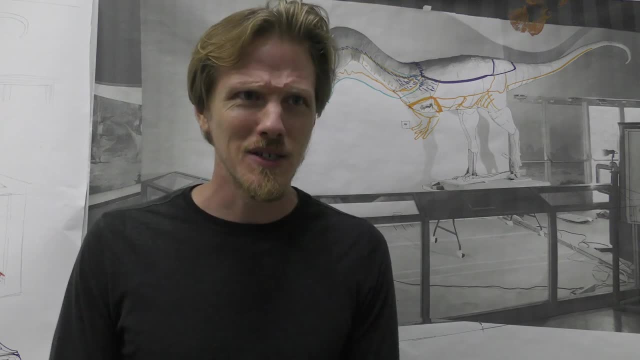 2020 meeting draws to a close in this strong, strange all-digital pandemic format, I was struck with this super last-minute idea to reach out to the paleo art community and ask people to send me one to three minute video clips introducing themselves and talking about. 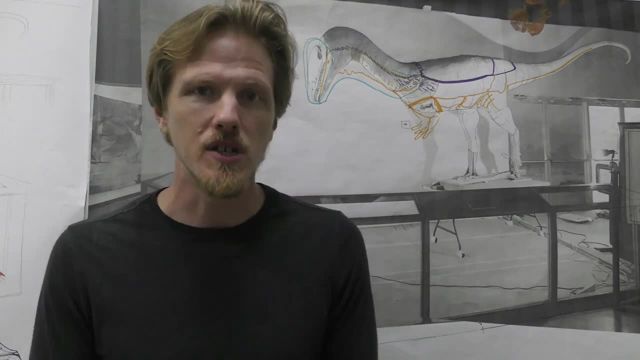 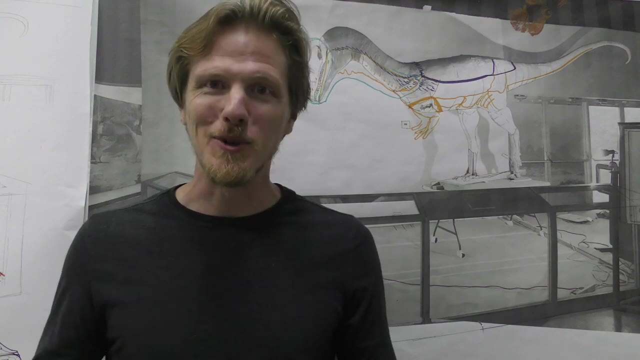 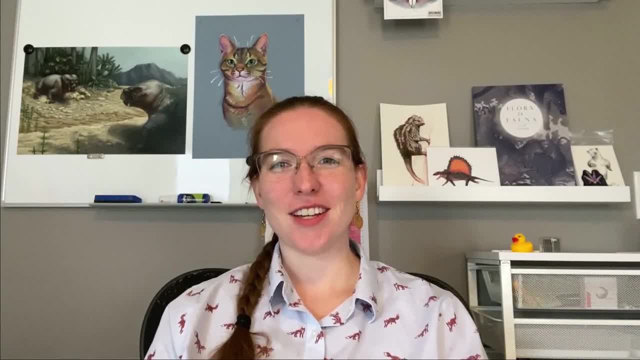 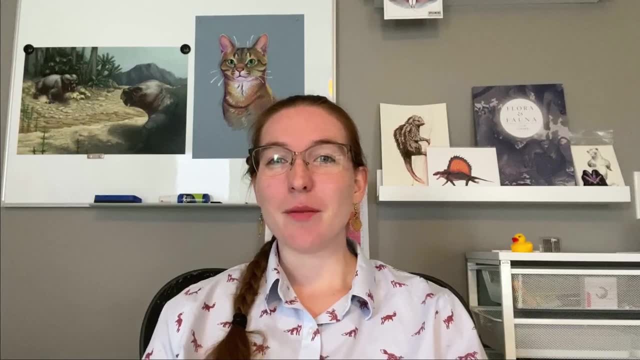 Hi, I'm April Neander and I'm a scientific illustrator and micro-CT research specialist working with Dr Lowe on mammal evolution at the University of Chicago. It might sound like an odd combination, doing scientific illustration and micro-CT work together, but I find that the 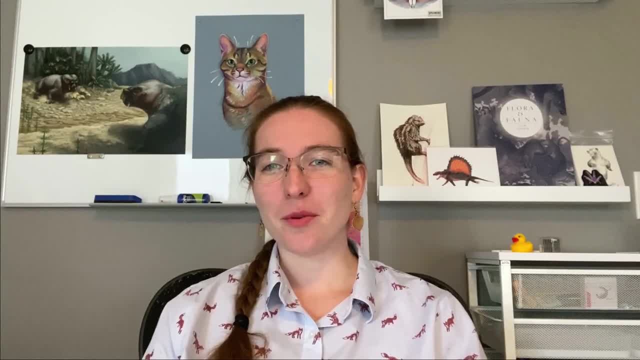 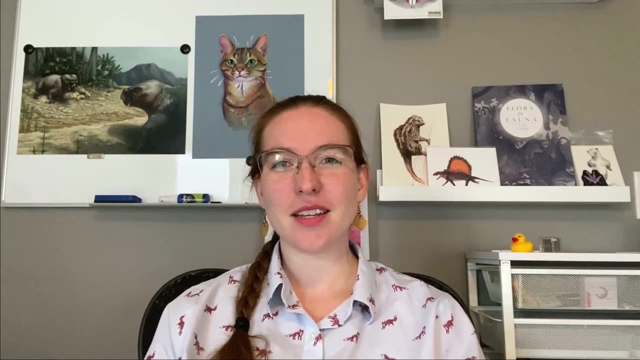 two have some really interesting synergy. For example, they both are really about the behavior of light at their core, which is an interesting topic. As an artist, I also have a great appreciation for some of the beautiful hidden structures within these specimens when I scan them. Today, I'd like to share an animation which was accepted as 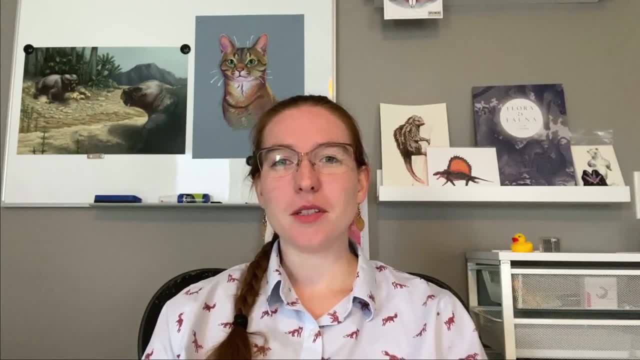 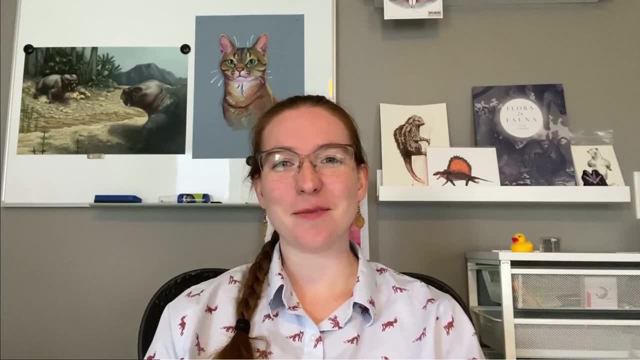 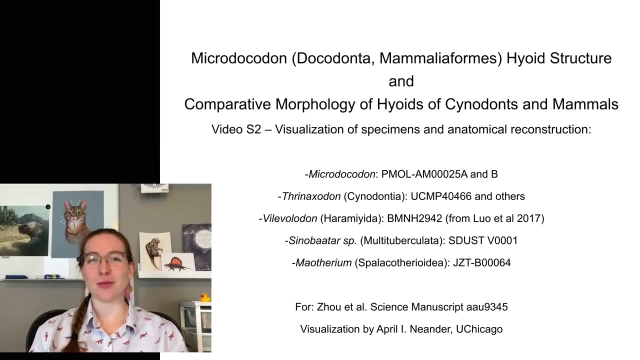 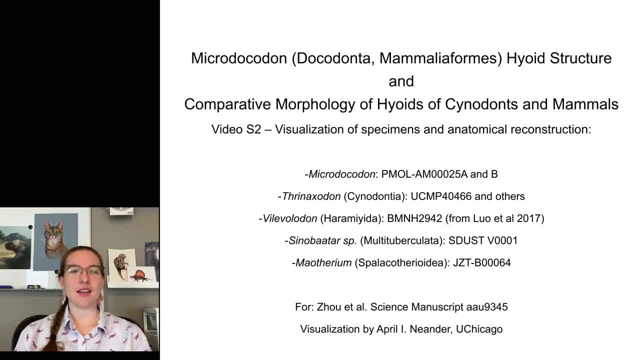 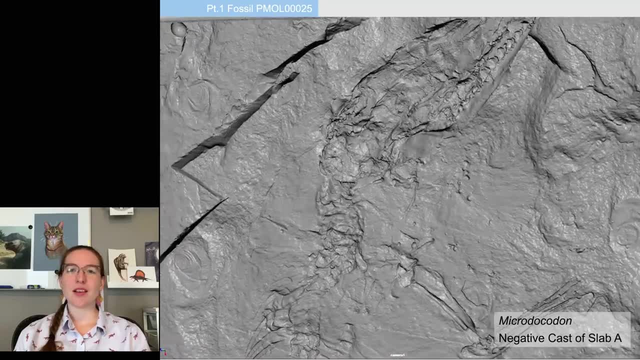 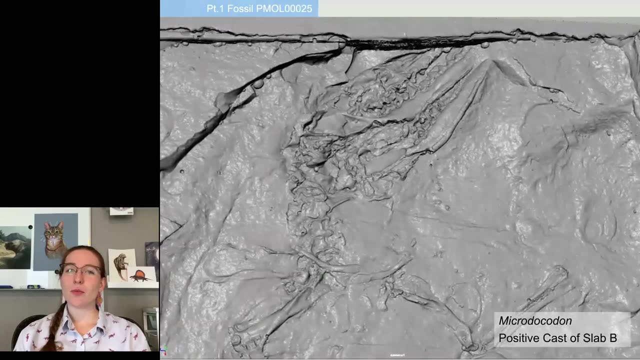 I'm going to show you how it's done. I'm going to show you how it's done. I start off the animation with scans of the primary slab specimens. A lot of the specimens that we work with are these flat slabs of pretty small mammals. It's common for papers to show 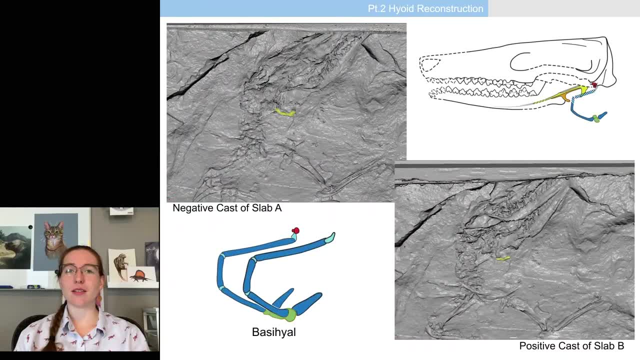 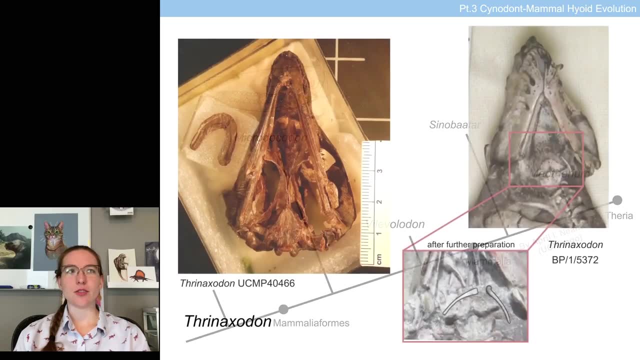 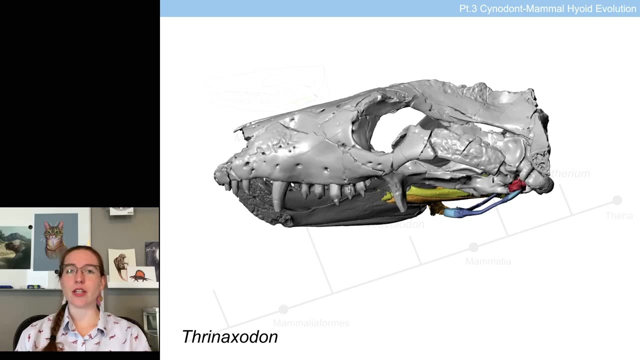 photographs of the specimens and outline the anatomy, but I thought it would make things a little more clear if I applied a glossy texture and tilted them. In the second part I introduced the parts of the hyoid and then in the last part, I placed the specimen within its evolutionary 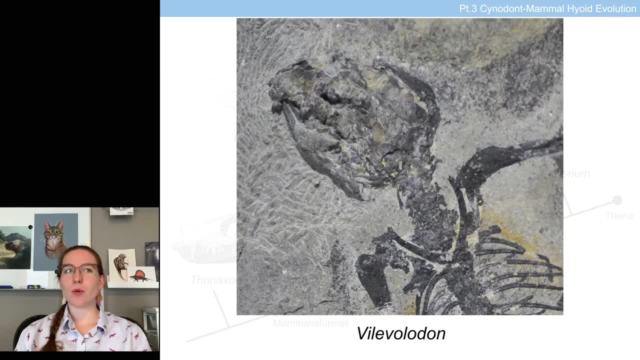 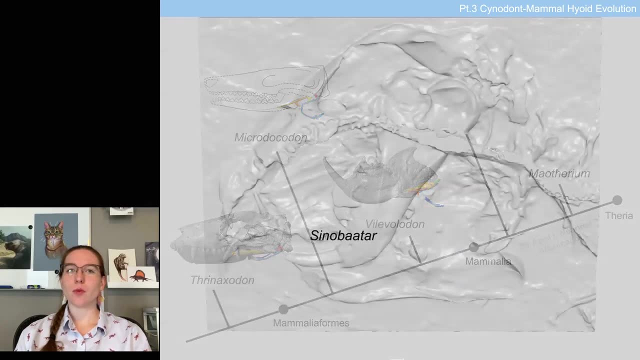 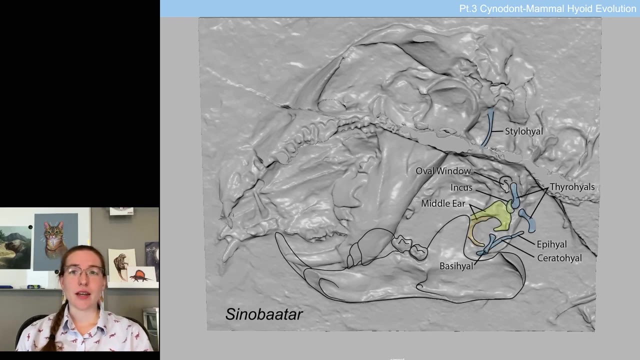 context of the mammal family tree. We want to tell the story of how the hyoids went from more reptile- like in therapsids to the more mobile and complex hyoids that we're familiar with in mammals today. These complex hyoids are indications that these animals were fully chewing their food before. 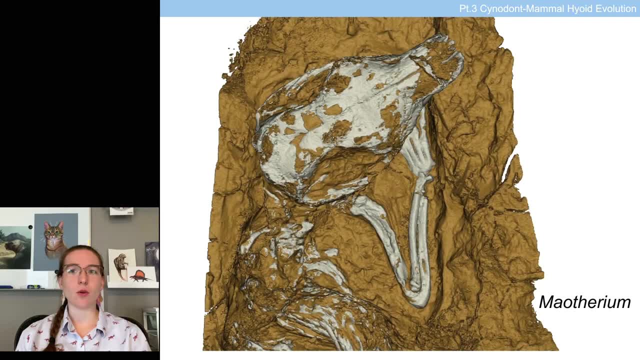 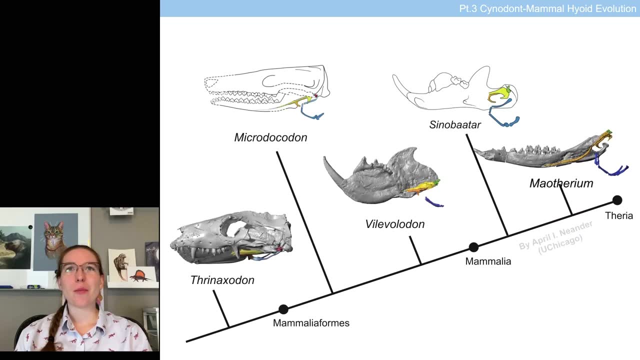 swallowing, whereas the hyoids were chewing their food before swallowing. whereas the hyoids were probably behaving a little more like reptiles and swallowing large chunks of food, The hyoids also show a possibility of the suckling behavior in these animals. These structures are so small and 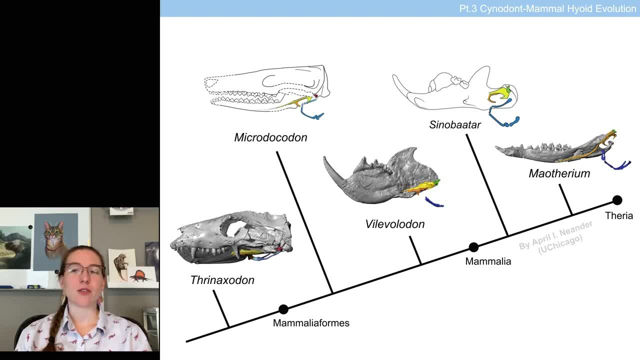 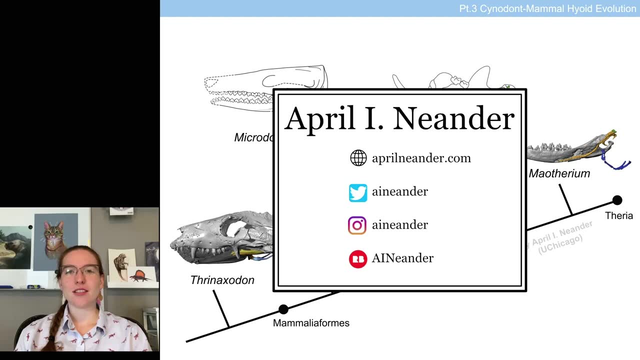 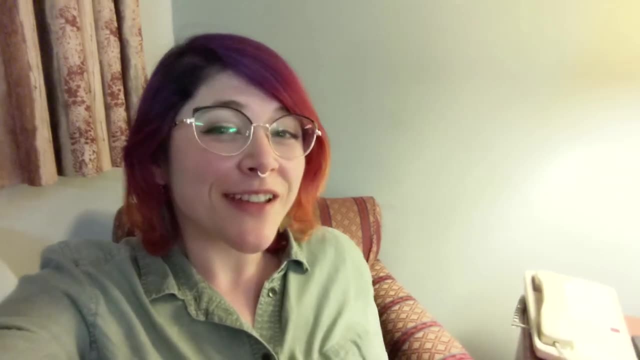 delicate that we would never have been able to describe some of them without microCT technology. Thank you for watching, and if you'd like to learn more, you can follow me at any of these locations. Hi, I'm Danielle Dufault and I'm a scientific illustrator at the Royal Ontario Museum. 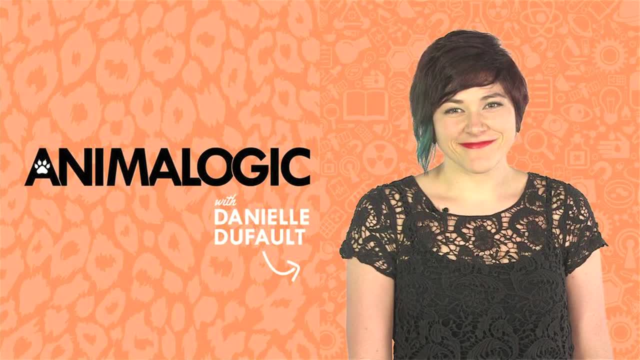 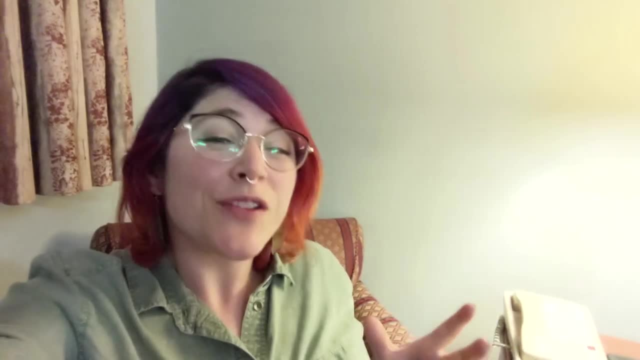 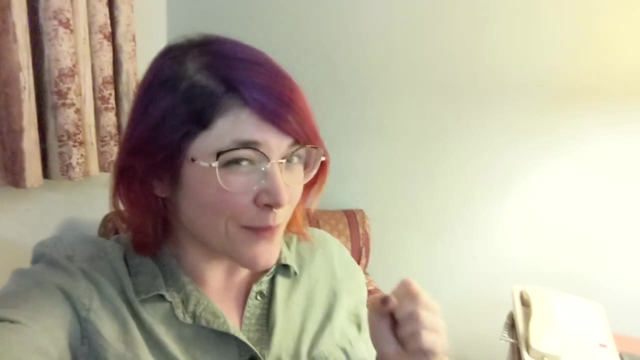 and host and illustrator for Animalogic on YouTube. When I'm not observing black bears during the salmon run on Vancouver Island or watching wombats engage in territorial kerfuffles on Moriah Island, I'm applying what all of my senses have taken in about this world, and applying it to the past. 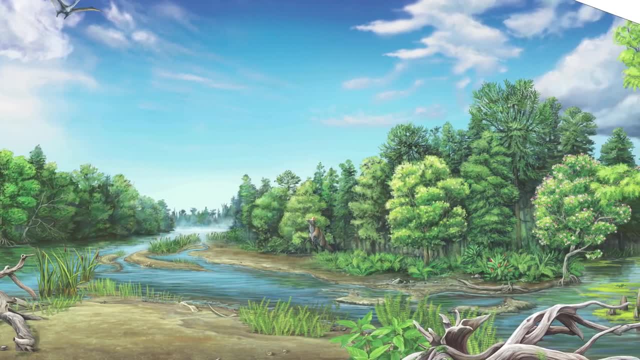 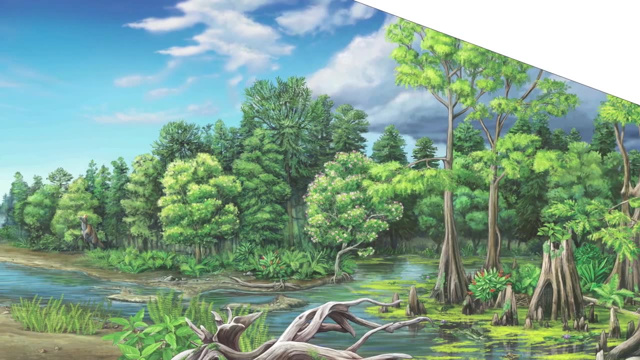 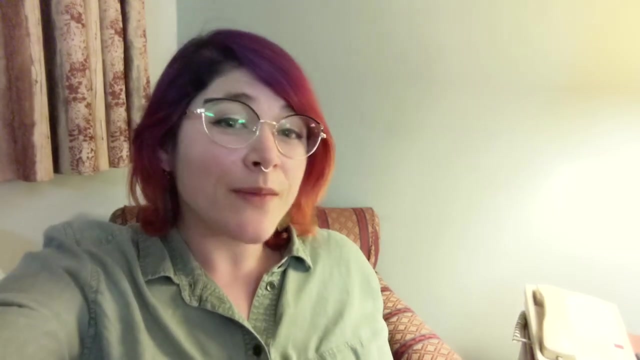 My heart lies deep, deeper in down through the many geological layers that compose this beautiful planet, and I firmly believe that the better we can understand the biology and ecology of the lifeforms around us, the better we can know the animals that have come before In recent times. 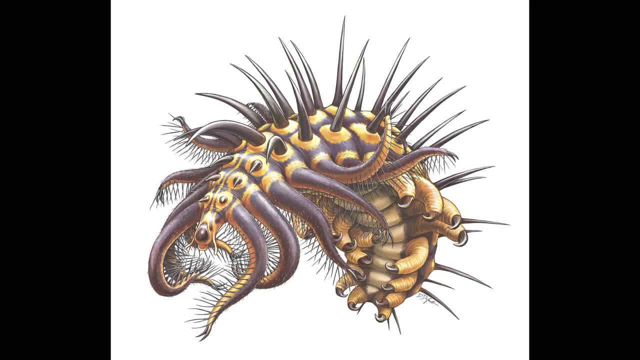 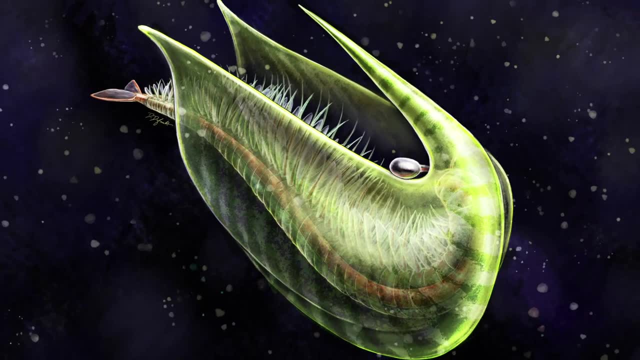 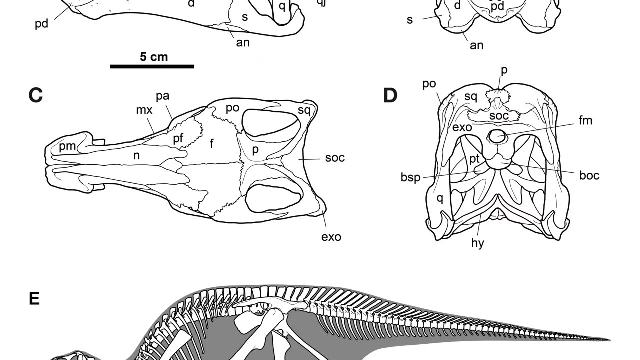 I've illustrated creatures from the Burgess Shale like Colenzovermus monstrosus with Jean-Bernard Caron and Fibulacaris nereidis with Alejandro Izquierdo. Further up in the Mesozoic, I illustrate the anatomy of dinosaur bones, create anatomical diagrams. 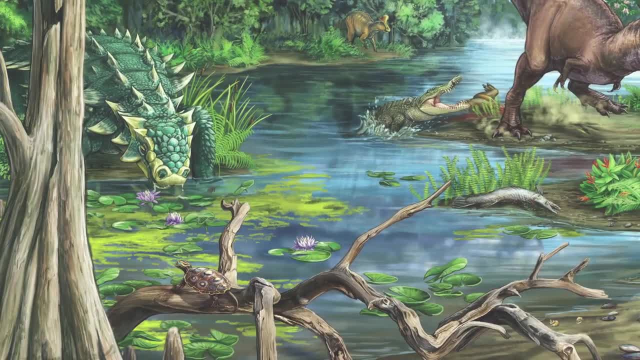 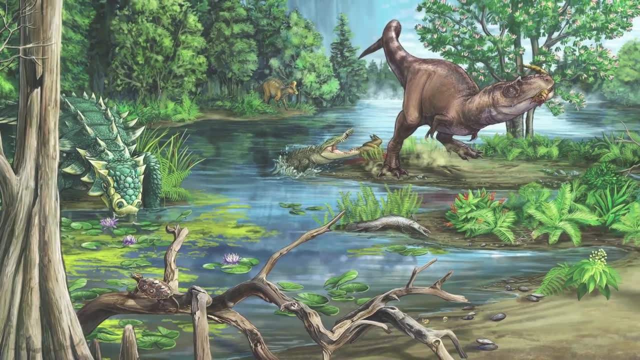 and reconstruct entire ecosystems in collaboration with Dr David Evans and his lab at the Royal Ontario Museum. As an example, I made murals for the exhibit featuring Zoolchroorivostator, a new ankylosaurid dinosaur from the Judith River. 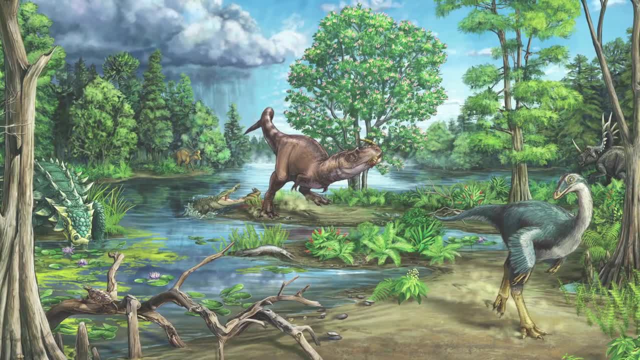 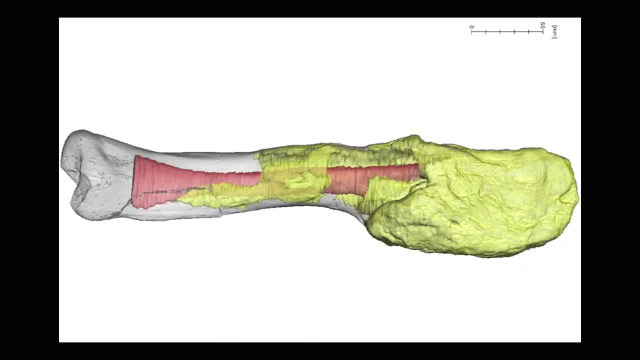 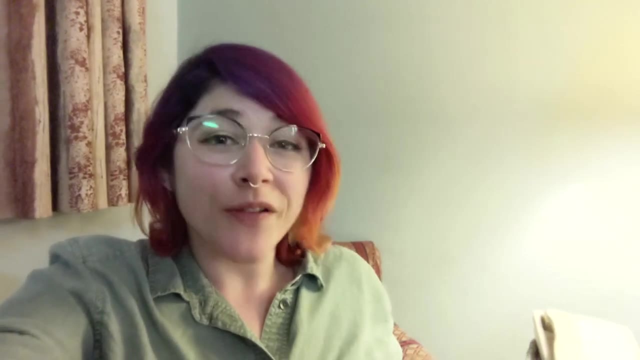 Formation with Dr Evans and Dr Arbour. I also work with CT scan data to visualize tissues like this incredible case of osteosarcoma in a very, very unfortunate centrosaurian dinosaur. For every step of the work that I do, I try to draw. 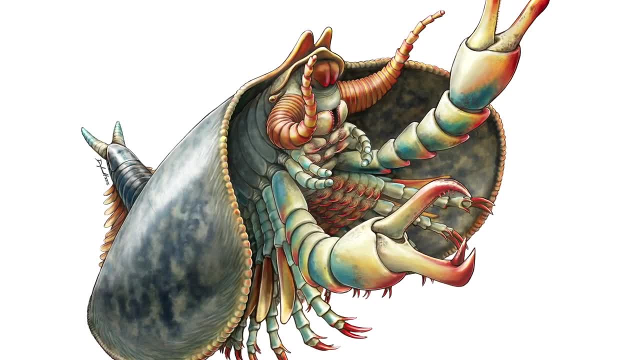 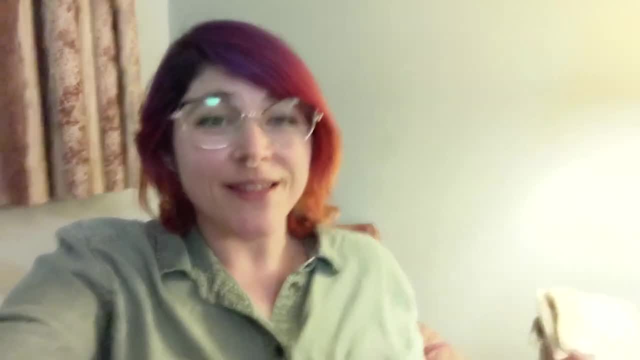 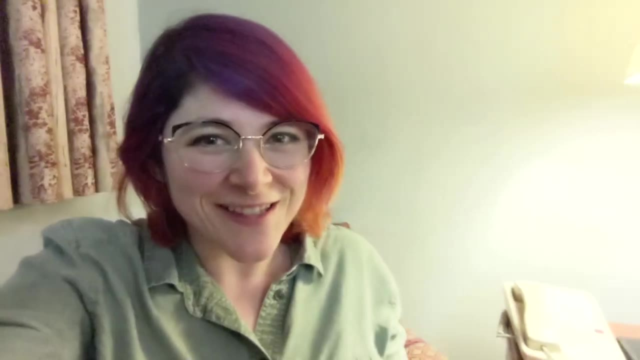 inspiration from the extant world around me, which is why I'm so engaged in communicating the wonders of the natural world in so many forms. I'm sad to miss SVP this year, but keeping my boots on the ground and observing the incredible diversity of Earth will surely inform my next piece. You should have seen the size. 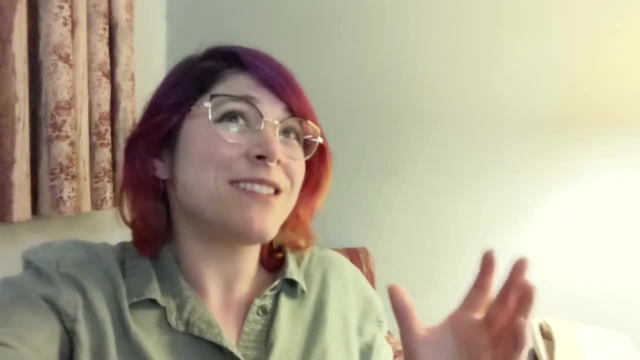 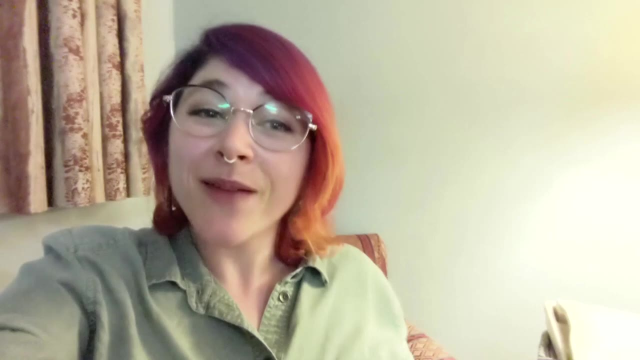 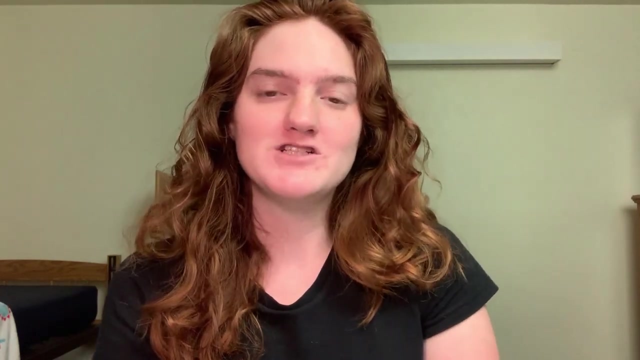 of the Iquacetum that I found earlier. It looked positively carboniferous. Gotta get back to scoping out some bighorn sheep in Jasper. but thanks for your time and attention. Cheers. Hi, my name is Tess Gallagher and I'm an undergraduate at Union College in 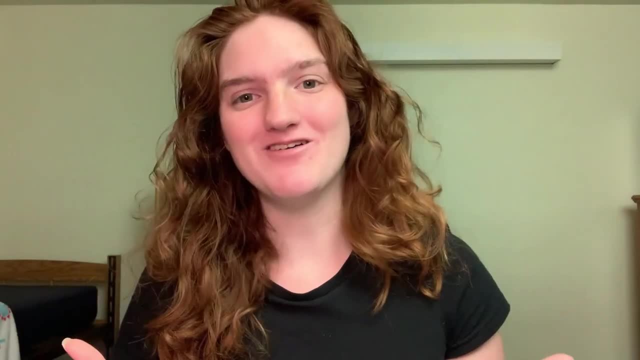 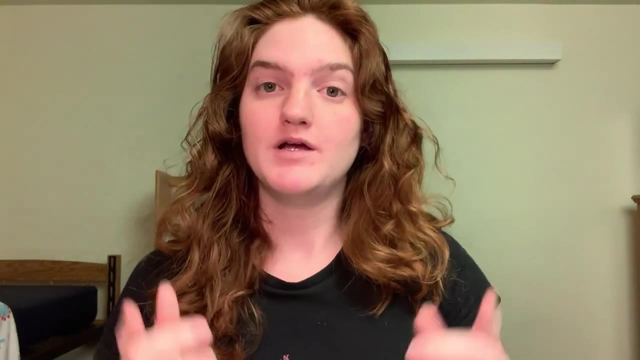 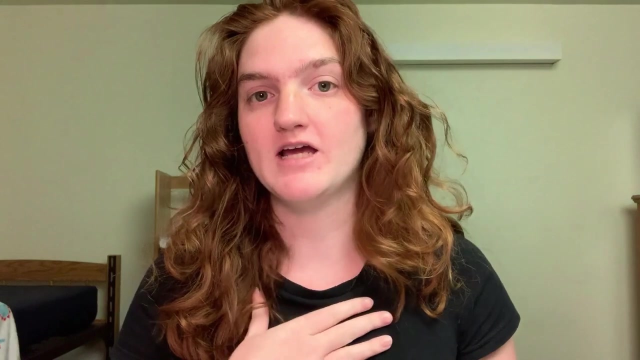 Schenectady, New York, and I'm also a paleo artist, so I haven't actually made anything for a museum or a paper yet I am actually in the process of working on a piece for a paper that I actually did the research on. It's not published yet. 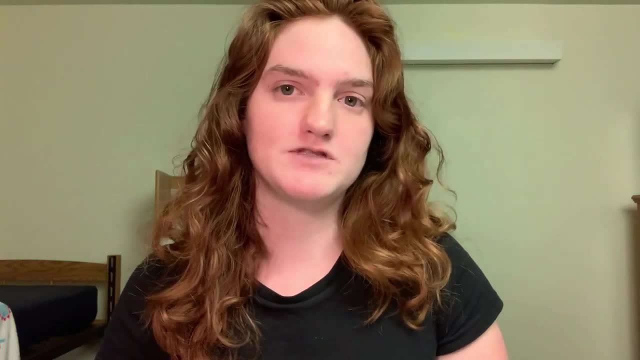 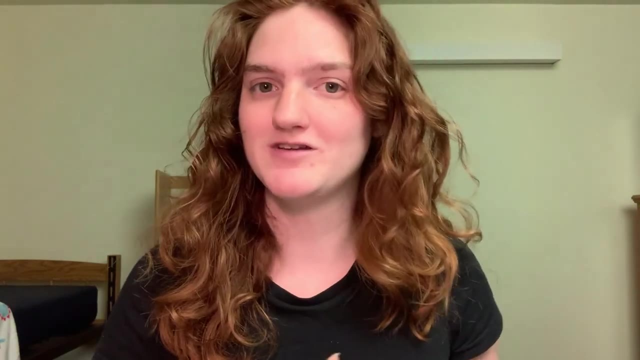 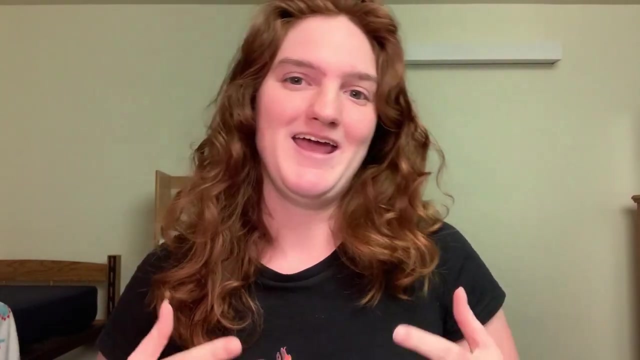 and that paper is on evidence of scale diversity in Diplodocus, SP from the Mother's Day, Quarry Montana, and that's also a poster that I'm doing for SVP, So I can't show you that artwork. unfortunately It's not done and not published, But instead I will show off this. 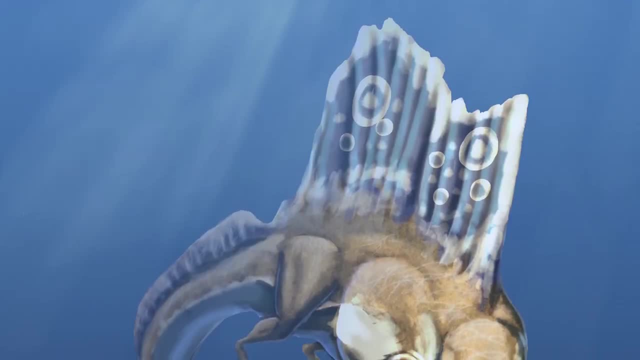 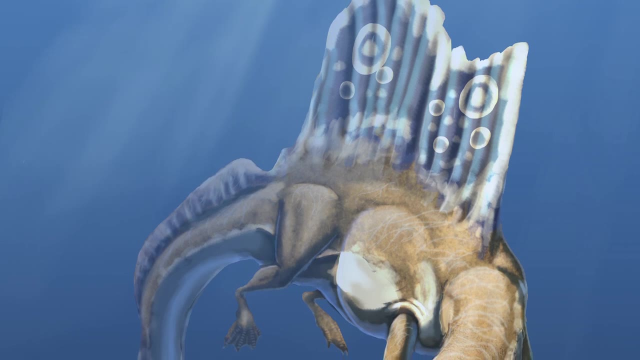 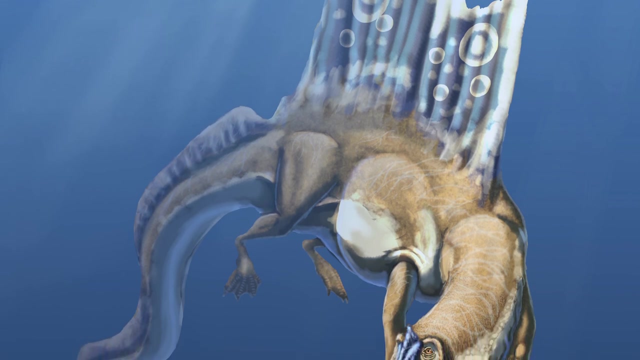 spinosaurus artwork I did this summer because I'm really proud of it and it shows, you know, I mean it's my favorite dinosaur, so of course I'm in love with it. but also I was kind of trying to experiment with a new kind of a. 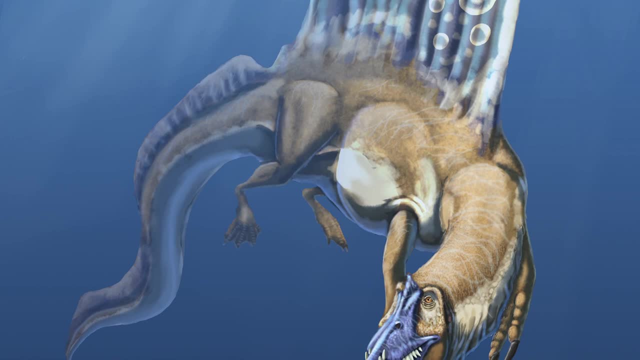 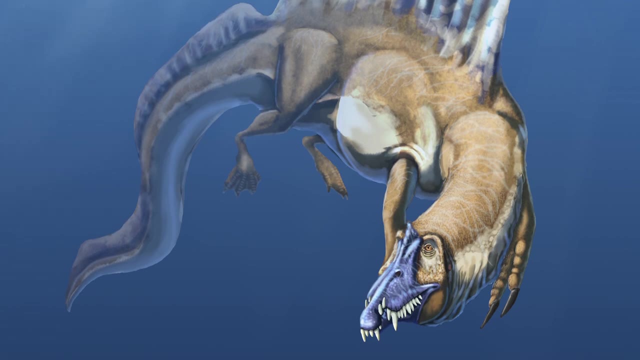 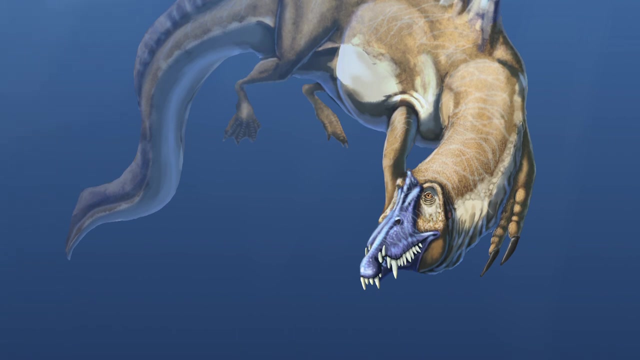 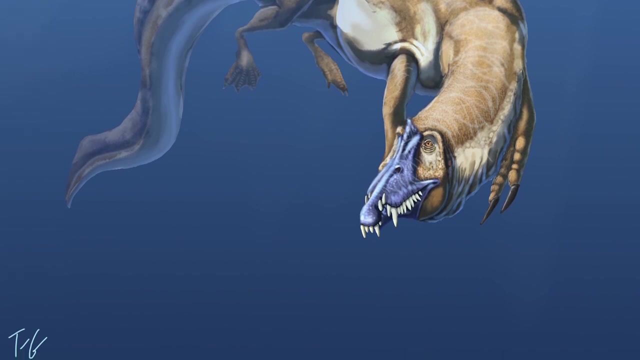 technique for doing scales, Because, uh, scales are kind of a bother for pretty much any paleo artist, uh, but recently I've been drawing- you know I like to doodle with pencil, of course- and I have found a way to draw scales. uh, they still look like individual scales, but it's much faster and it doesn't cramp my hands. 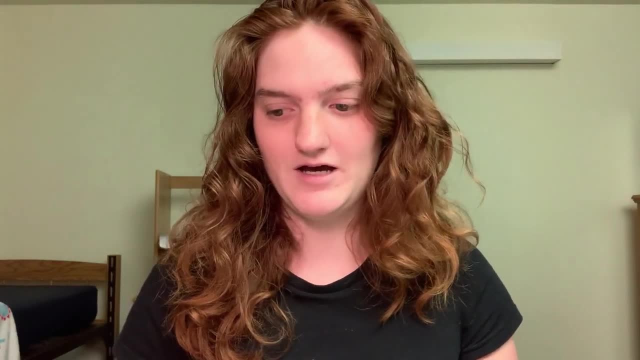 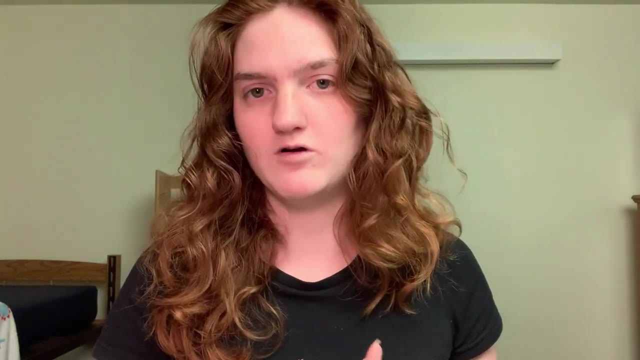 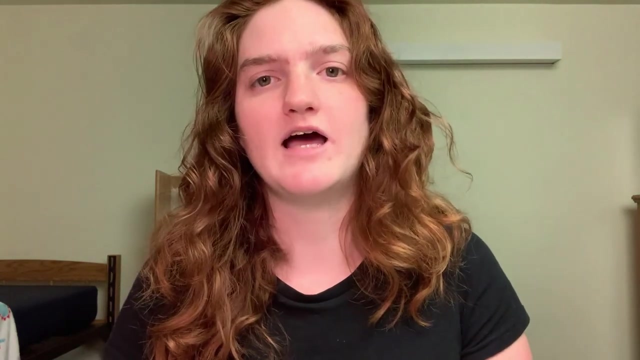 so I've been trying to experiment with, uh, my, my pencil art style, but also, uh, my photoshop art style. so also the the artwork- uh, my Spinosaurus artwork- that was done in photoshop. so I'm trying to like play between the two different styles and see if I can find a way to make it easier. 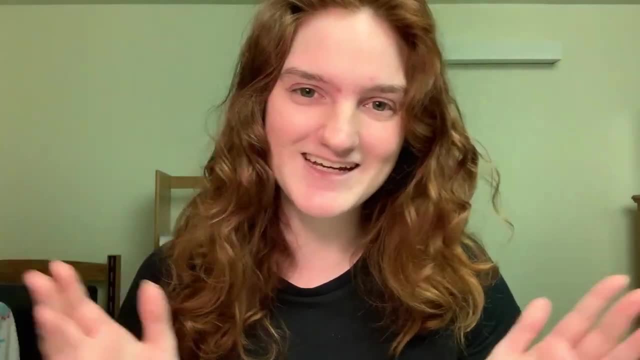 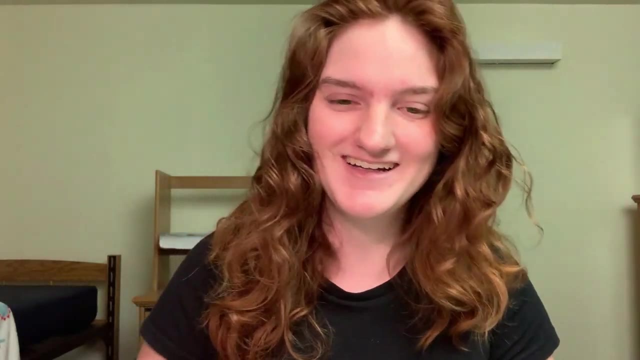 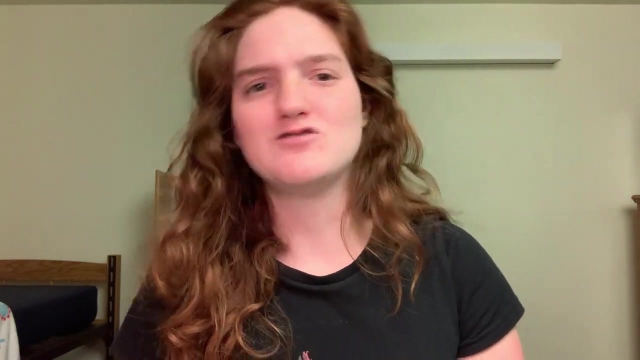 to draw individual scales that won't cramp my hands, um, because I definitely need it for, uh, my other artworks that I'm doing for my paper. um, this artwork, uh, I believe it took me anywhere between five to eight hours. uh, it's usually about how much my artwork takes for me to do, at least in photoshop, um. 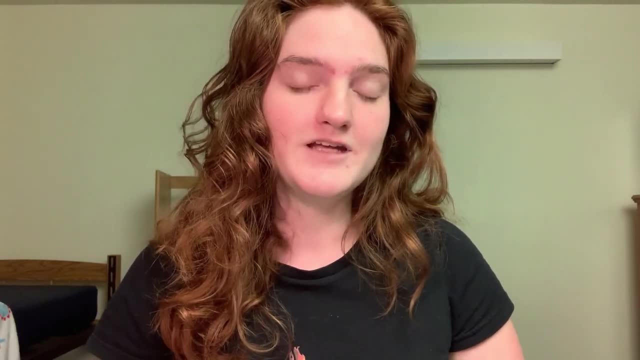 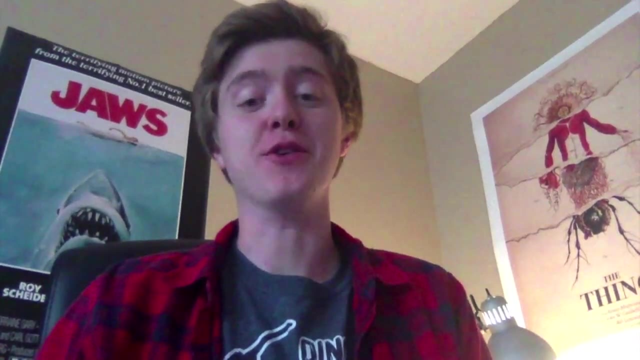 and uh, yeah, that's all I have to share. thank you, hi. paleo people. my name is Henry Sharp, I'm a paleo artist and a paleontology student here at the University of Alberta, and I'm going to be talking about a piece I did about this time last. 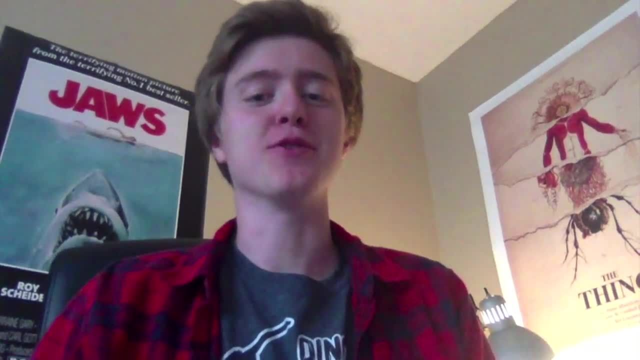 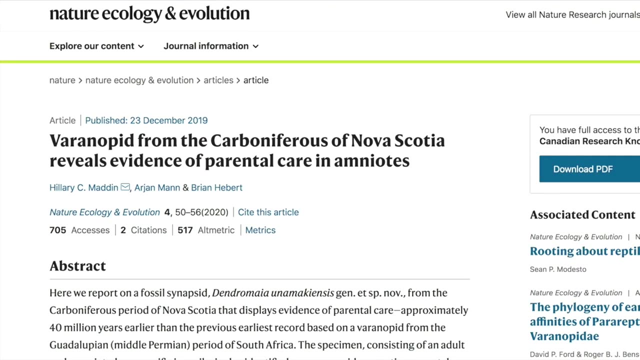 year for the the I'm Dr Hilary Madden at the Madden Lab at Carleton University here in Canada on an animal called Dendromya. so Dendromya is a varinopid reptile from the Carboniferous and it was preserved right next to a younger individual, probably of the same species and given other 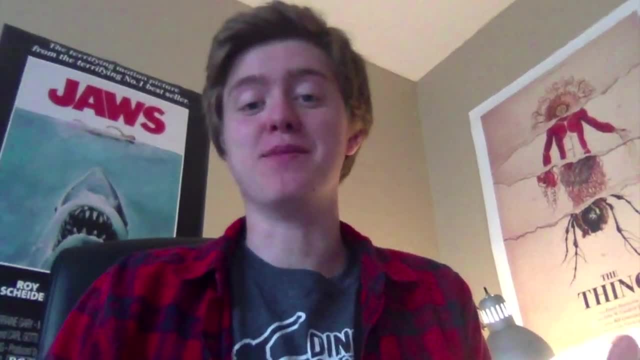 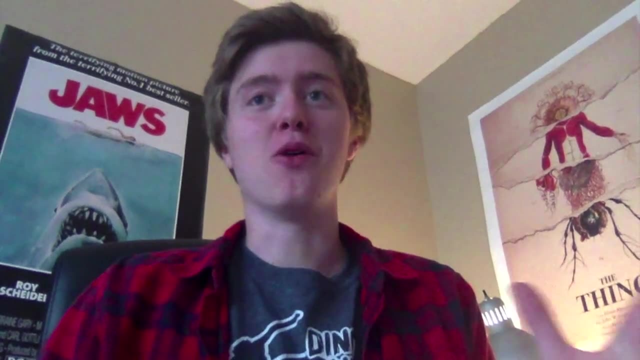 fossils from this family. it probably indicates the earliest example of parental care, which was really cool. I was stoked to work on it and I'm going to be going through a bit of my paleo process. so I started off with uh going through old sketchbooks and looking for 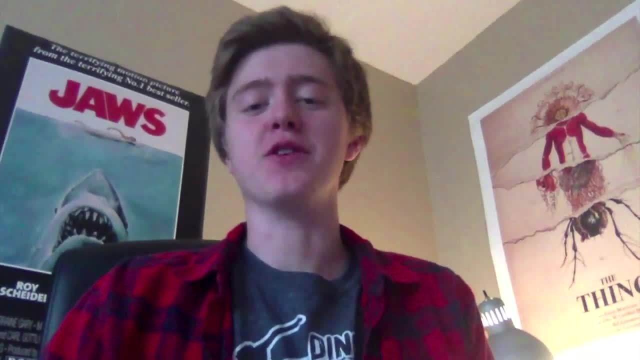 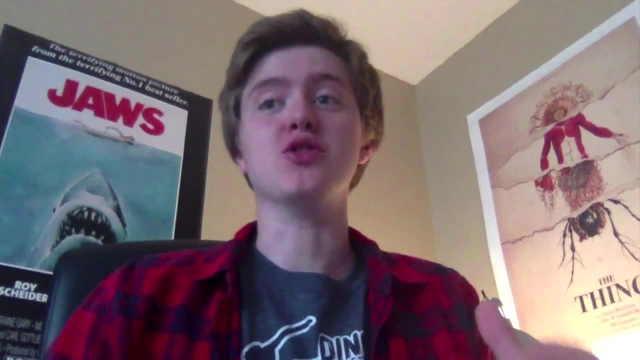 drawings of reptiles about that size, and so I found a few of uh katanasaurus that I really liked, and they were really liked by the client too, so that was great. then I moved on to the plants, because carboniferous plants are very different from plants today. 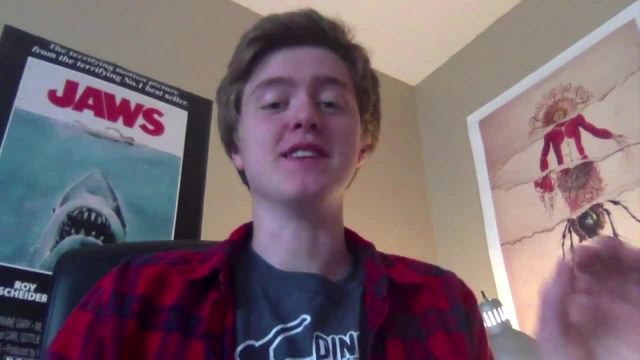 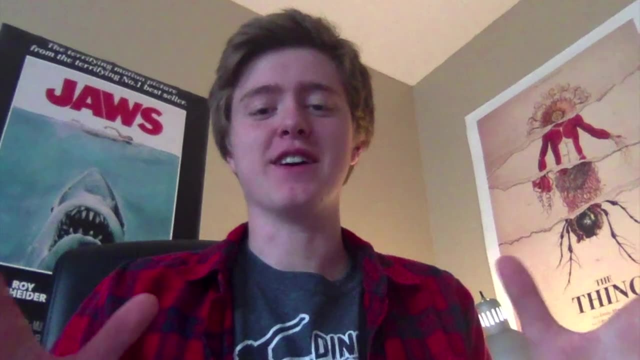 and I was able to sit down with Dr Eva Koppelhus, who is the paleo botanist in chief here at the University of Alberta- really cool person- and she showed me around all these different uh collections of carboniferous plants from that area, so I was able to take some. 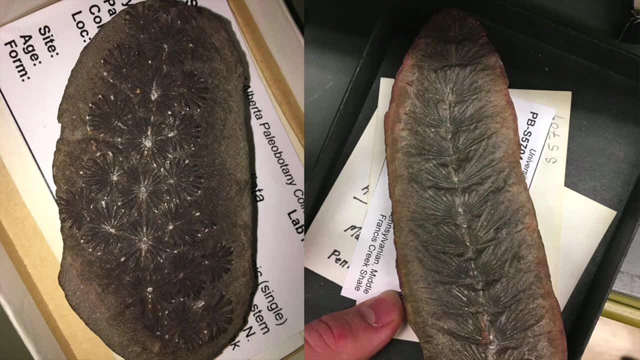 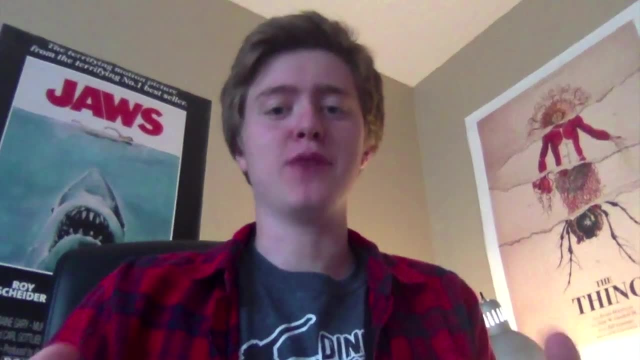 some pictures, do some sketches and find out that some of the plants- horsetails- are actually still found here in Edmonton. So I went down to the river valley here and I picked a few dead ones and kind of mushed them up a bit, put them next to my laptop and I was able to draw from. 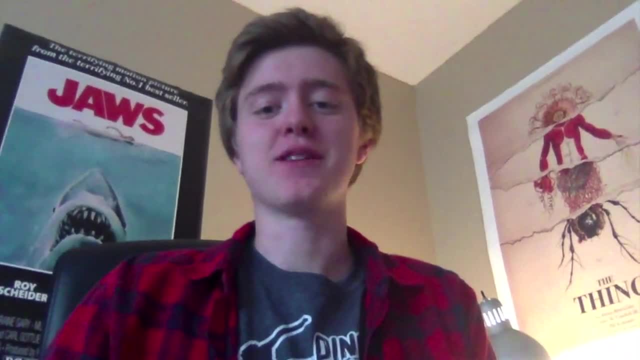 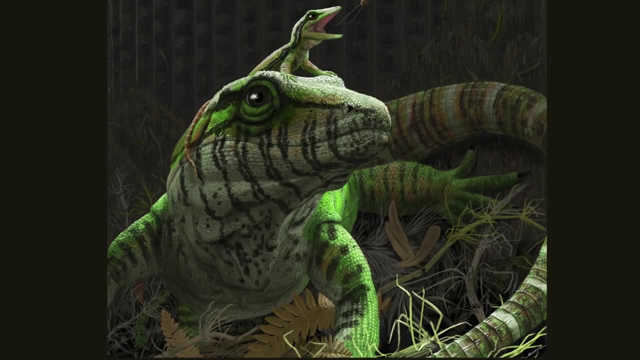 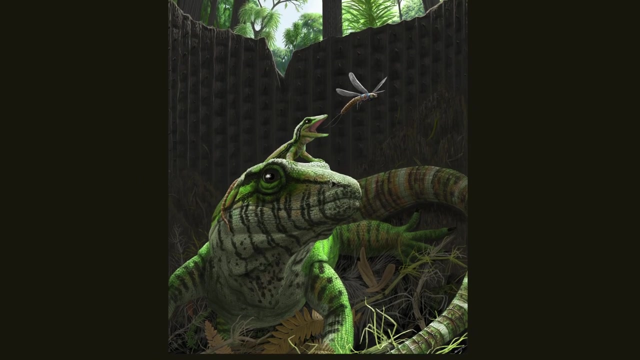 life to kind of get that cool den, look for how these animals were nesting. Because drawing from life, it always makes your art a thousand percent better when you're drawing something from your imagination, as paleoartists have to do So. at the time that I finished this, it took me two. 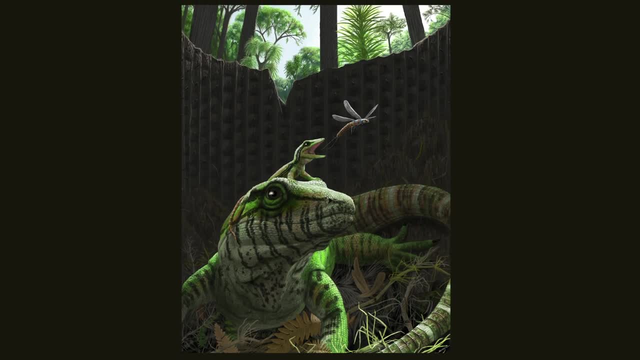 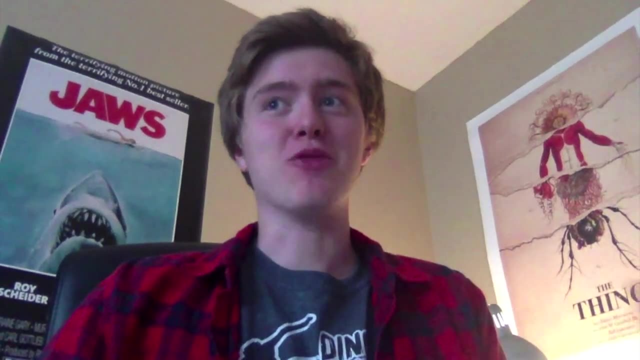 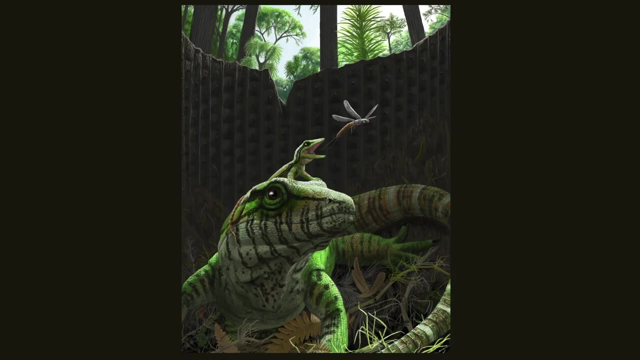 weeks to finish this. It was a really tight deadline but it was so much fun. The Mandalorian was coming out and so a lot of people were stoked about Baby Yoda and were kind of hypersensitive to cute baby reptilian things, And so when this came out I think that that probably contributed. 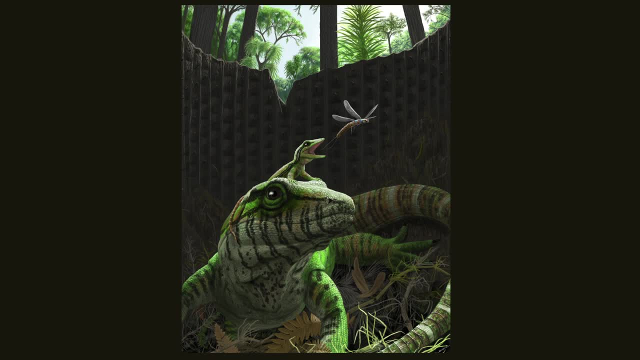 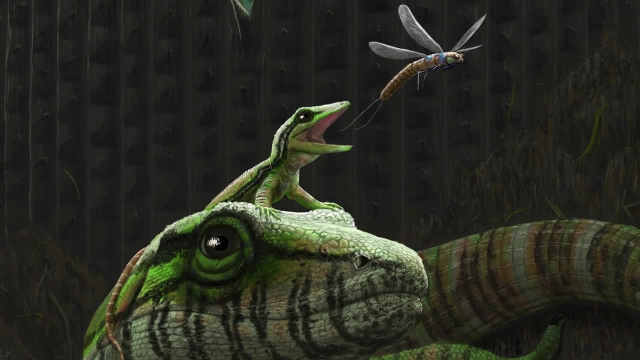 to the vast amount of coverage that this discovery got, Because, of course, we have the little dendromia sitting on top of the adult's head trying to catch an insect, And it looks pretty cute. It was intended to look pretty cute. 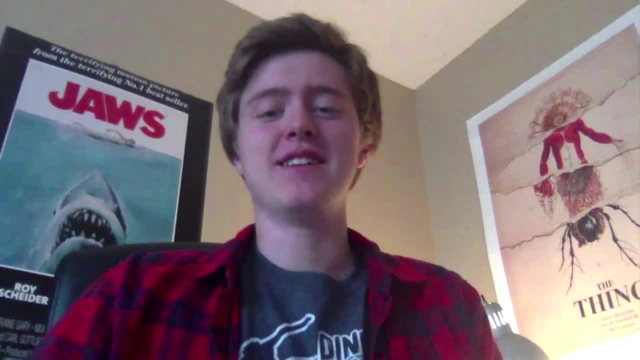 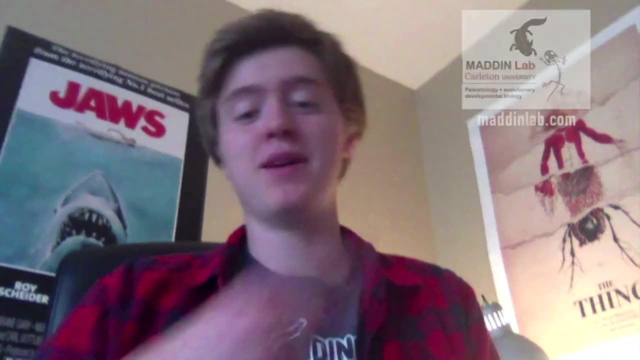 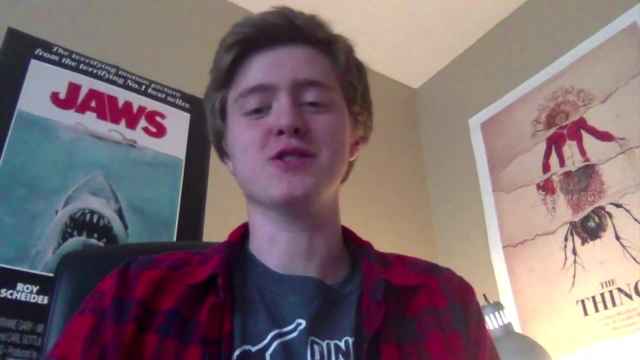 And, yeah, it probably contributed to the hype over dendromia, which was amazing. It was a tremendous experience. Check out the Madden Lab. Here's their website. They do some amazing stuff. They're a group of amazing people and I'm so fortunate to have worked with them, Thanks. 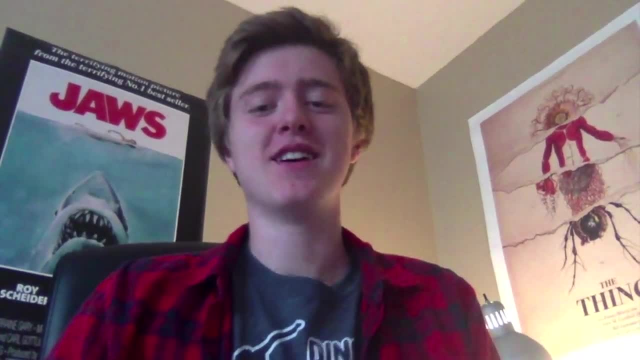 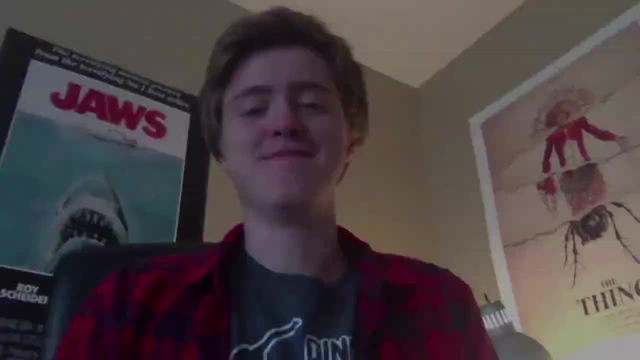 Brian For this opportunity. This is really cool that you're doing this and I can't wait to see what other paleo artists have for this. So yeah, thank you, Take care. Hey, so I'm Dr Brandon Peacock. I'm the curator of paleontology at the Idaho Museum of Natural 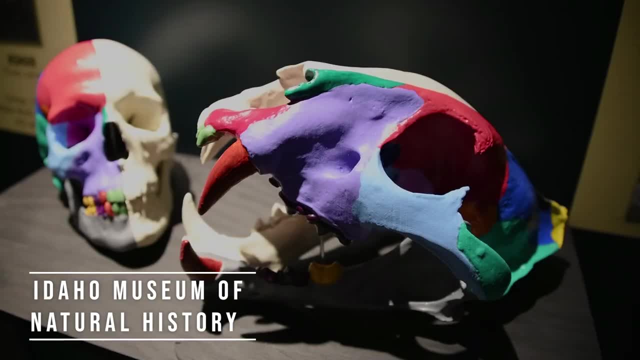 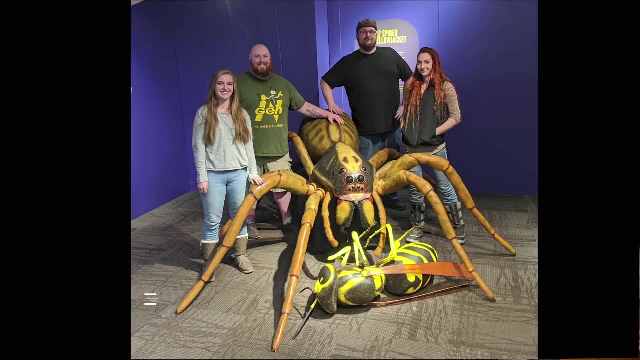 History. We're standing here in our newest exhibit called Skulls, which shows off so many of the specimens we have here. So we're talking about things like bones and fossils casts, but also a lot of things created in-house by our artists in the Idaho Virtualization Laboratory that we've 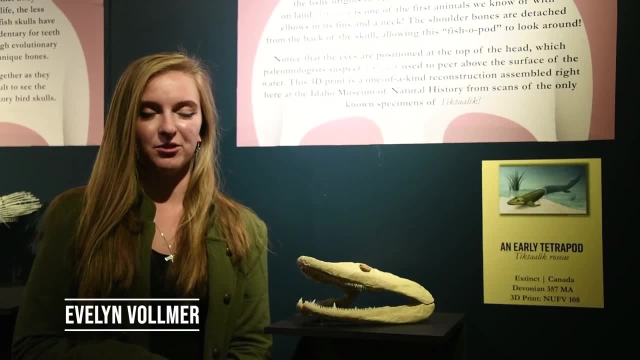 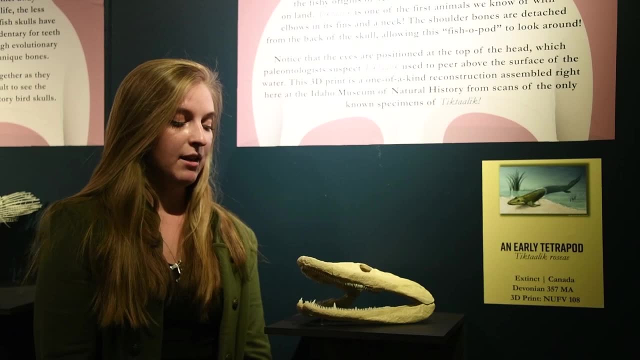 done in 3D printing. Hello, I'm Evelyn Bomer and I work at the Idaho Virtualization Lab. I got to 3D model this little Tiktaalik for the exhibit. It is actually based on the fossil material, but I did a process that. 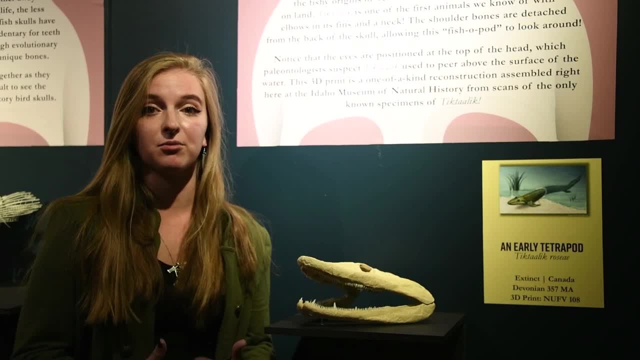 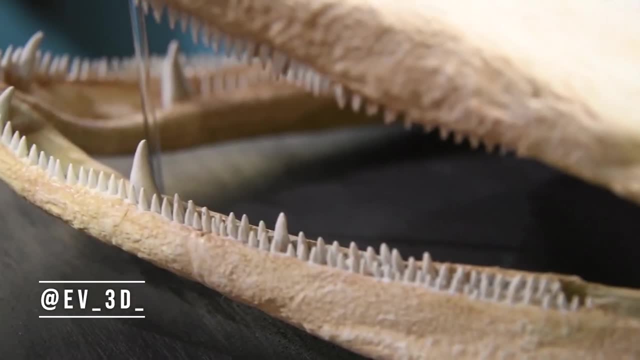 fixed the broken material and makes it whole again. This is the first one in the world of this, so it's a pretty amazing process and it was a lot of fun to do. If you're interested in seeing more of my work, I actually have an Instagram at EV underscore 3D. 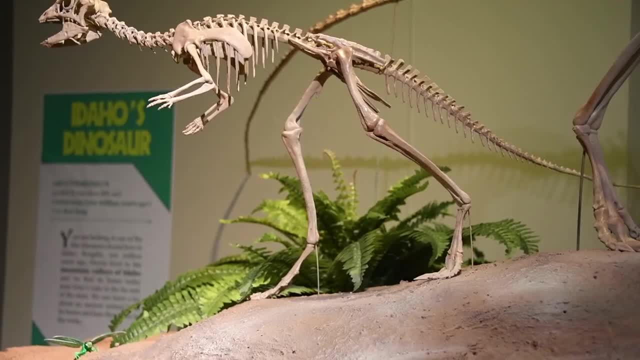 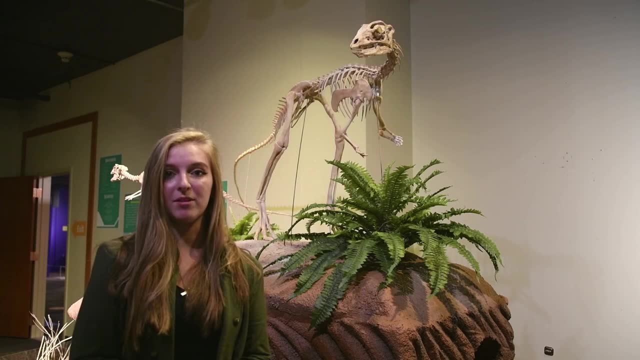 This is a Rictidromyus, Idaho's dinosaur, and we actually got to 3D model this with some students at the Idaho Virtualization Lab. So one summer we had a bunch of middle school students come in and they got to 3D. 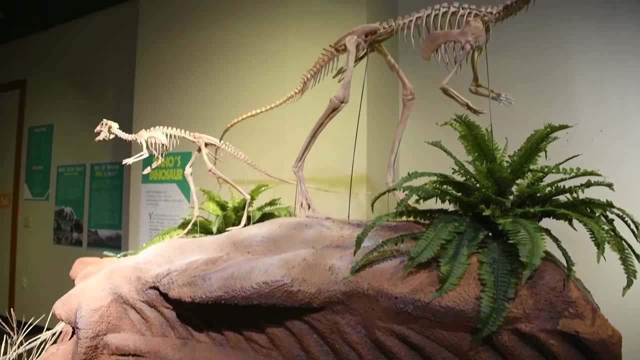 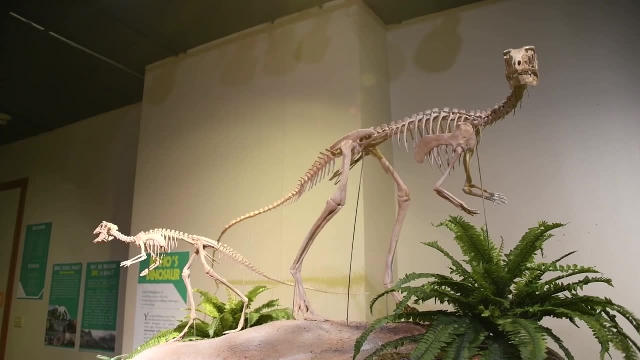 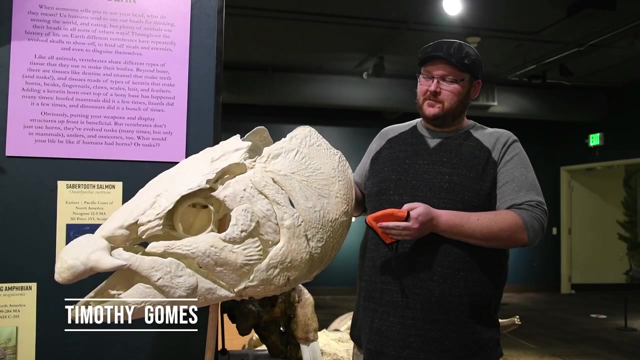 model the bones of this and then we printed it for display at our museum. We modeled this completely from scratch and we used reference material from the bones that have been collected in Idaho, but this was a complete digital sculpt. I'm Timothy Gomes. I'm the one that sculpted this saber-toothed. 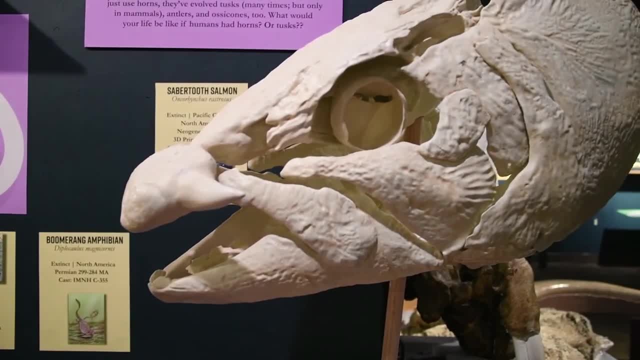 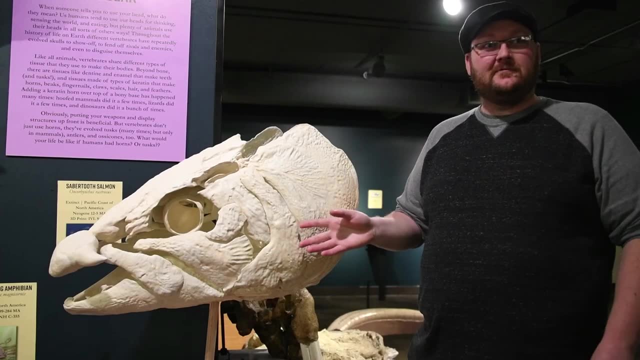 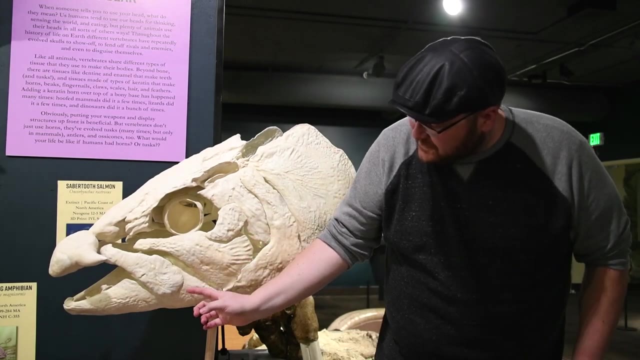 salmon skull. This is based off of essentially research data. One of the interesting challenges I had with this is essentially a lot of these pieces are connected with tissue so when I modeled and printed this, this is actually done in multiple pieces which we then found little loopholes and sections I can connect. 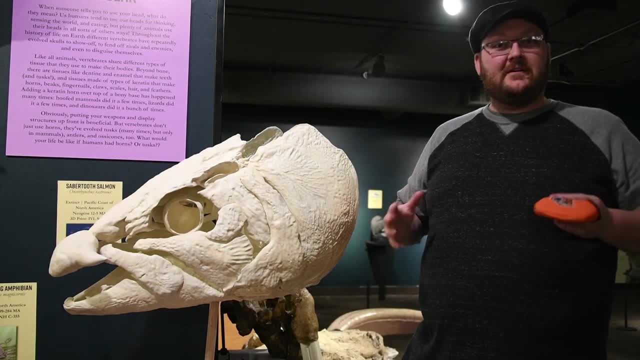 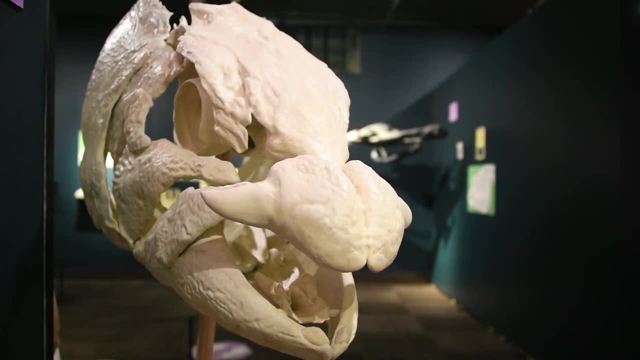 them with glue or just make little connection areas that I can put them all together. This is roughly the size of the biggest specimen found. This was based off of CT scan data. So of all the pieces in the exhibit, this one's actually one of my favorites. So this is this saber-toothed. 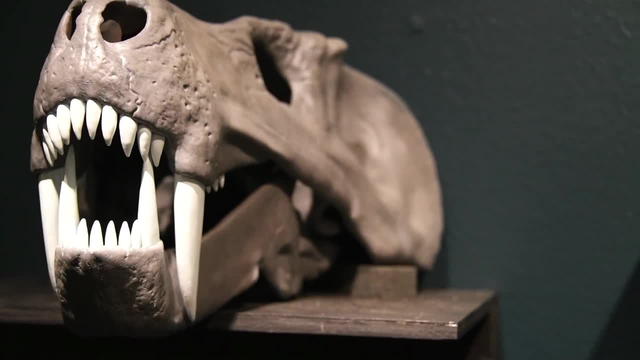 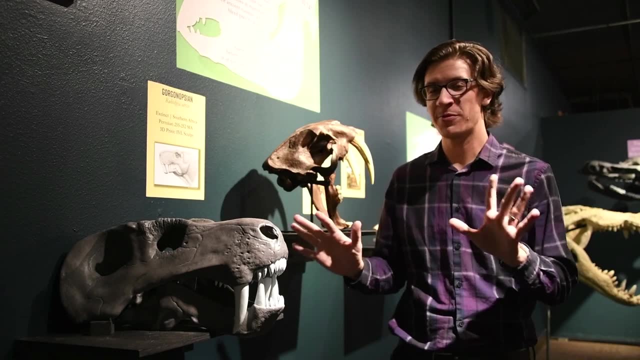 predator from the Permians before dinosaurs, a Gorgonopsian. It's actually one of the animals I do my research on that I found in the field. This gorgeous specimen on display now was sculpted totally from scratch by the head of the IVL, Jesse Pruitt, and so he and I, and 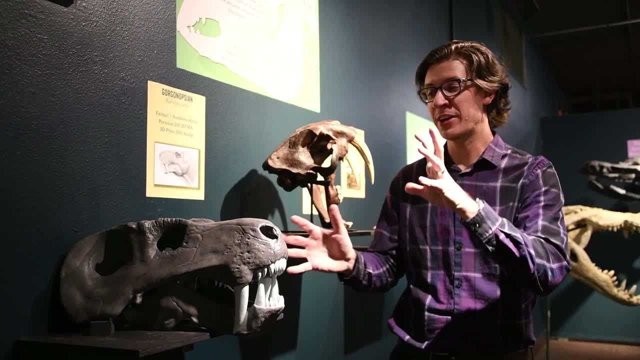 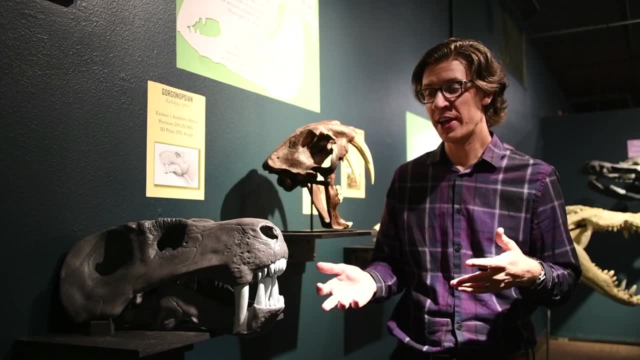 actually other scientists all worked together to digitally create this beautiful, beautiful reconstruction that's also informed by you know, scientific figures And now people when they come in to see our exhibit and they see more familiar saber-toothed animals like Smiledon or the saber-toothed marsupials. 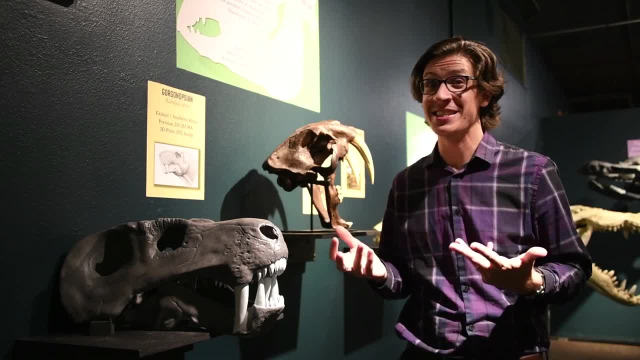 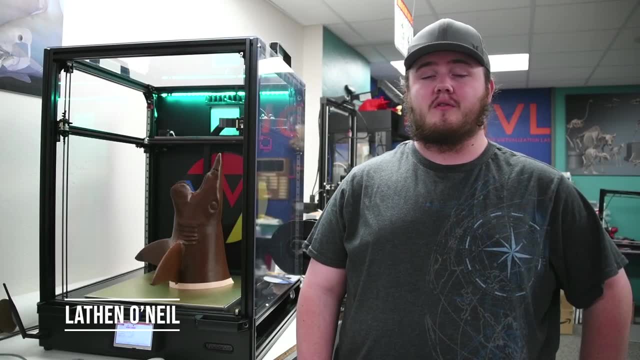 they can see this animal from the Permian that most museums, at least in the States, don't really have good specimens of, and it's so awesome. Hello, my name is Latho O'Neil and I'm an intern here at the Idaho Virtualization Laboratory. 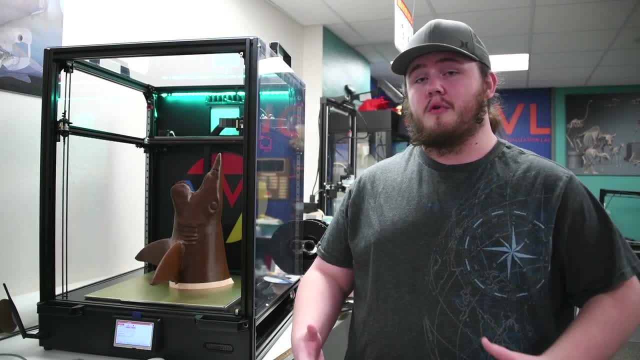 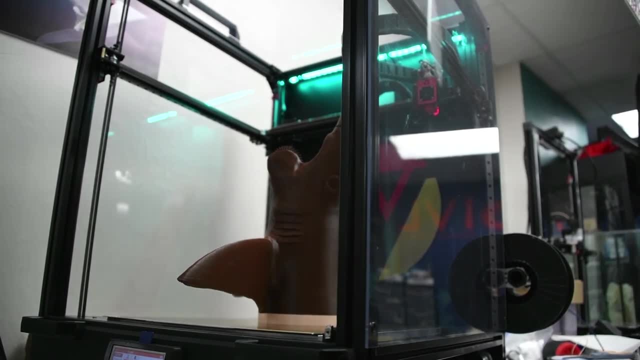 So what we did for the exhibit is that we worked on post-processing for 3D models. This post-processing was done on 3D models made from 3D printers, such as this one, which uses plastic filament to make 3D models such as the one you can see on the bed here. 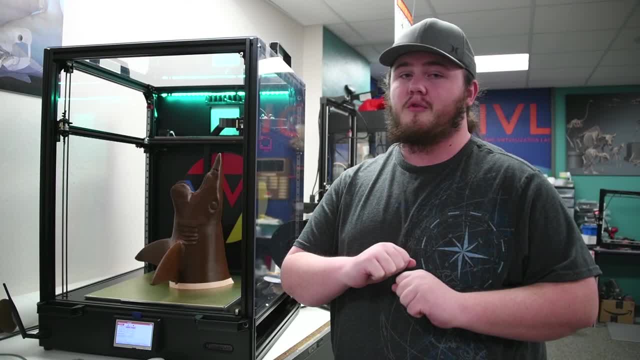 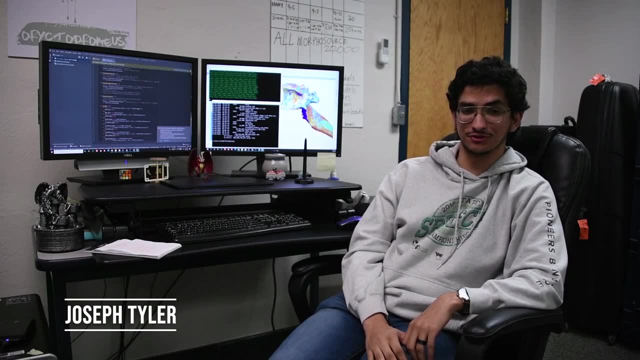 And then also we made 3D models for the smaller ones with a lot more detail involving the resin printer. Hi, I'm Joseph Tyler. I'm a computer science major here at Idaho State University and I work for the Idaho Virtualization Lab. 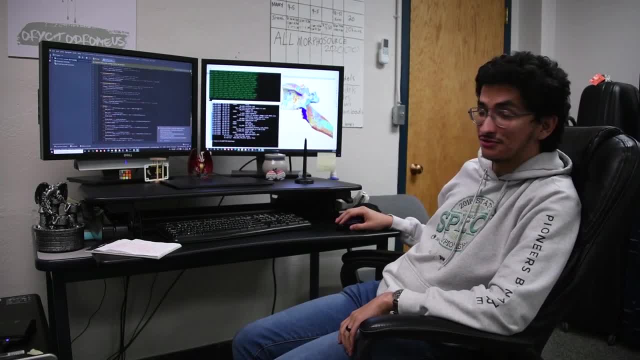 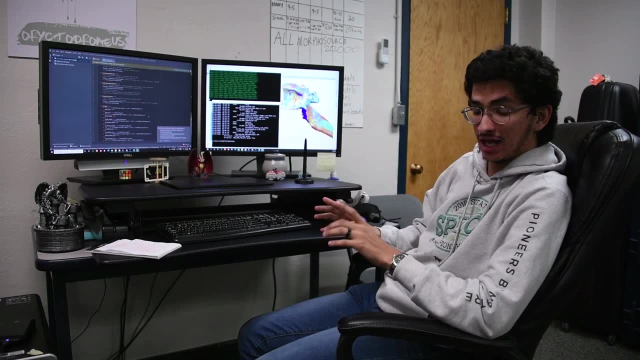 I'm a CPI here and, as you can see, I spend a lot of time on the computer and rewriting programs and codes so that we can help transfer our models up to an international database that anyone has access to. More recently was the skulls exhibit I was participating in. 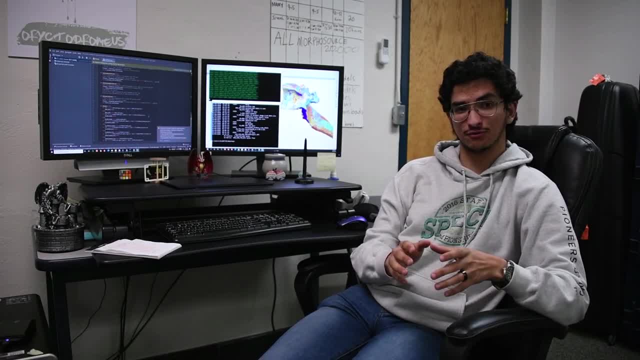 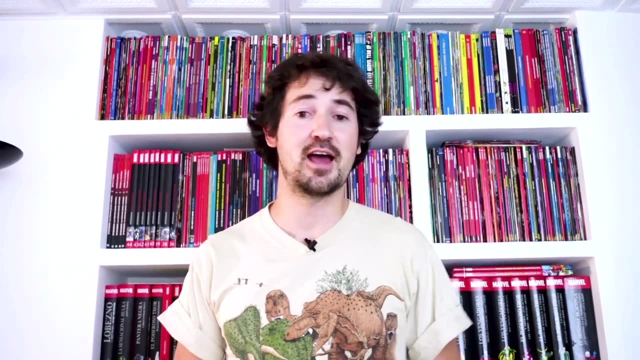 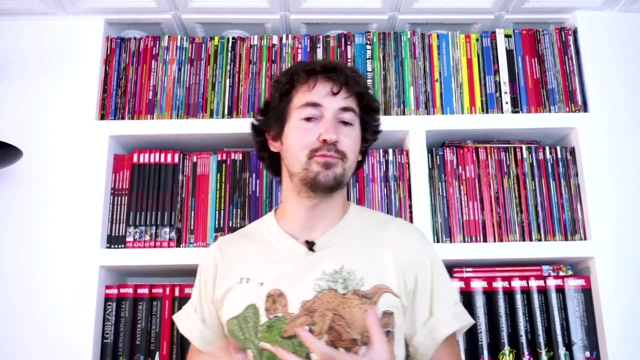 and assisted in the fabrication and creation of one of the biggest exhibits at this museum. Hi everyone, I am Dr Jesús Realid and I am a post-doctoral researcher at the University of Granada in Spain, but I am also a paleo artist. As a paleo artist, I'm happy to have produced some 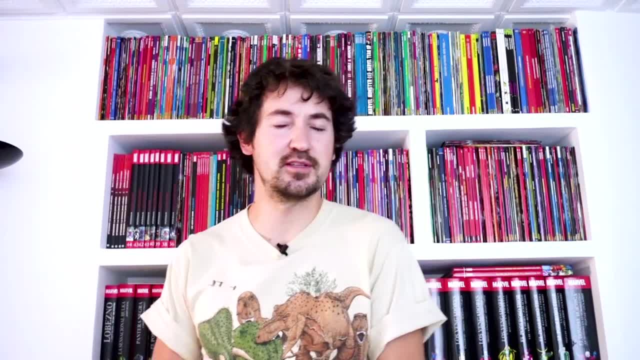 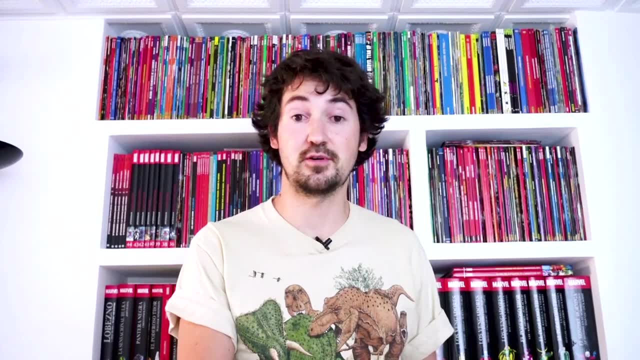 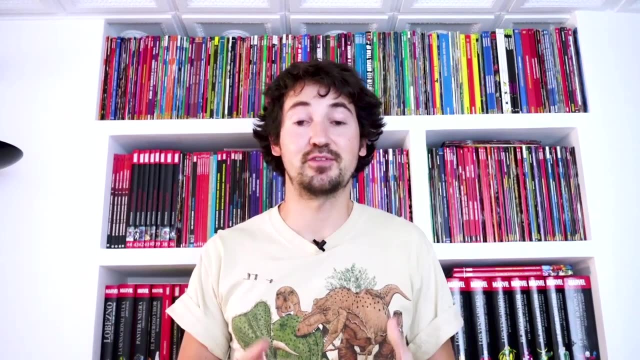 artworks, for books, for short movie series about paleontology on YouTube and also for some displays in museums at the Natural History Museum of Valencia in Spain. Today I want to introduce you to my favorite piece of work that is called the Path of the Iwanodon. it's an 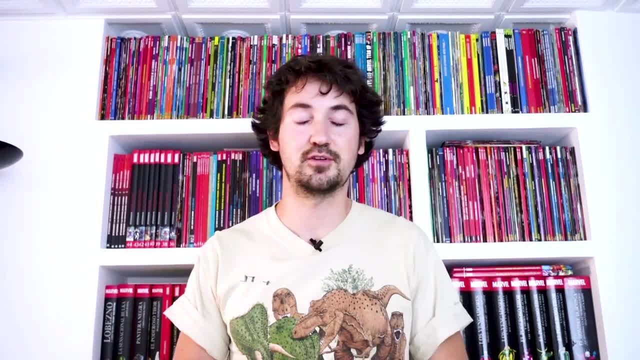 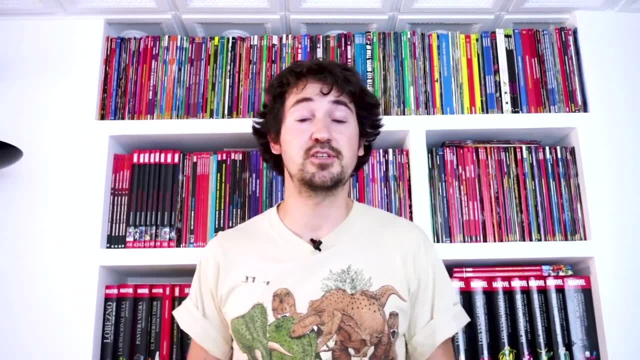 illustration I prepared for the geology and paleontology museum in Hamburg in Germany. It had been also recently published in a book about the history of life published by the editorial McGraw-Hill in Spain. This is an illustration which was done directly on paper. 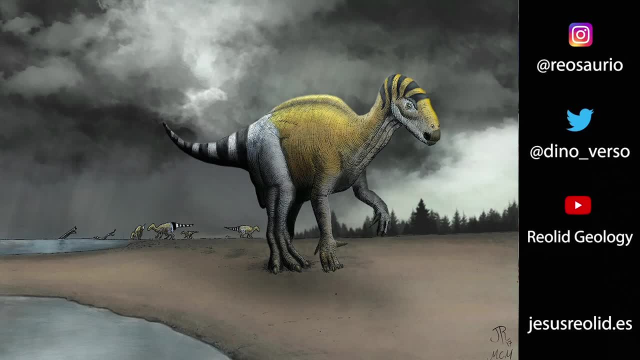 then I used inks over the original draw, over the original sketch, And when the ink was finished, then I digitalized it and color it in Photoshop with the help of my wife. And for what was done so it was for a display in the entry. 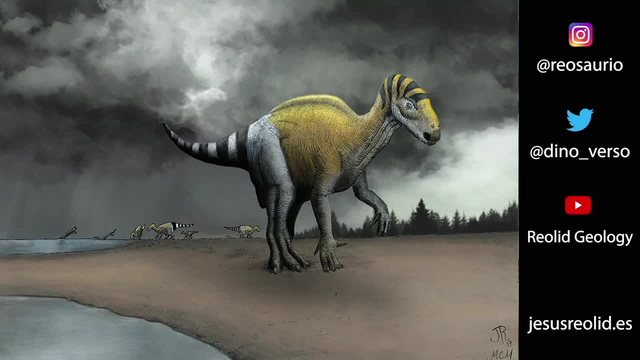 of the university building where the Geological and Paleontological Museum of Hamburg is placed, And this display is a huge rock plate like few meters long that is full of Iwana Dom footprints. You have different footprints of Iwana Dom. 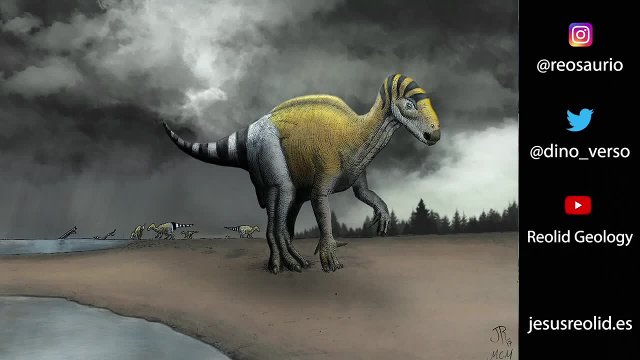 in different directions And also you have impression of the raindrops. So that's made me think about the environment. So I was thinking in a pathway where a lot of individuals were working, probably during the migration. So that's why I decided to put some different individual. 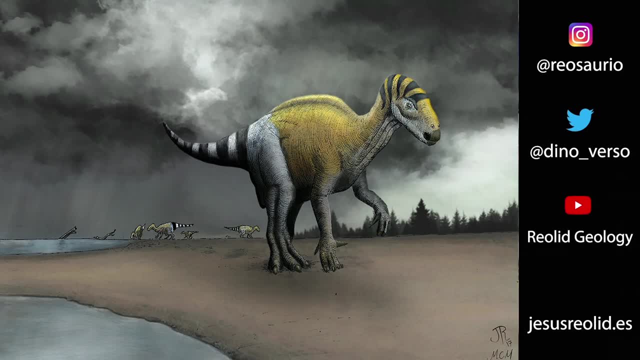 in the background, not only the main one. So I placed an Iwana Dom in the front side because I want people to understand how the animal was, And also I decided to have the Iwana Dom walking in a rainy day because of this raindrop. 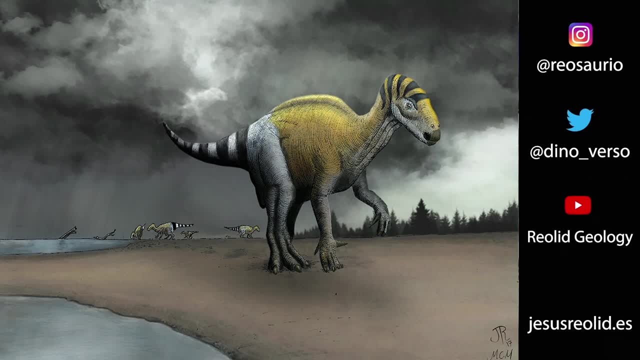 So it's cloudy in the bottom ground And then for making the figure of the dinosaur popping up out of the background that is really sandy and gray because of the clouds. then I decided to give some really bright colors And then I decided to use the one. 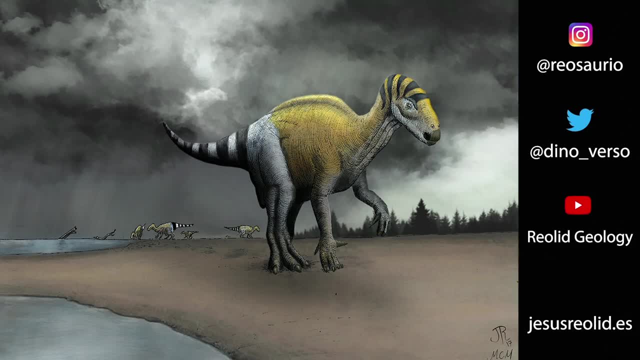 of my favorite bird, the hippo, And I think that the final result is kind of nice, So I hope it's going to be great, hope you like it and if you want to know about my art or find some more information, and contact me. 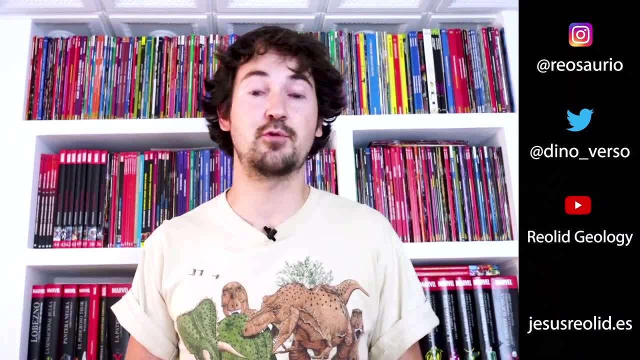 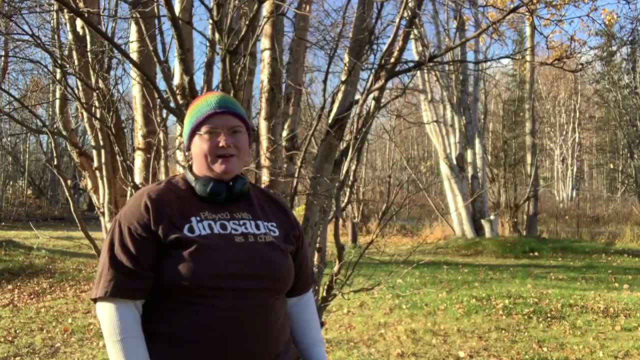 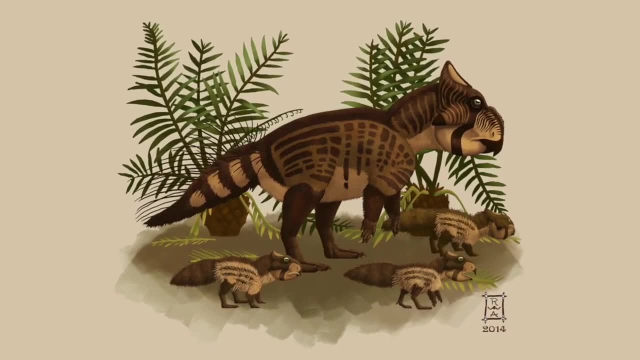 for anything. here you have my social media and my website where you can contact me at any time. thank you for your time. cheers, hello everyone. this is raven amos, paleo artist, and this is buster. buster is, of course, just a nickname for a small sheep-sized relative of triceratops. 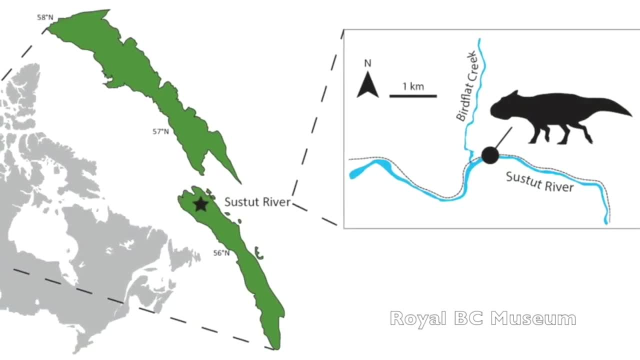 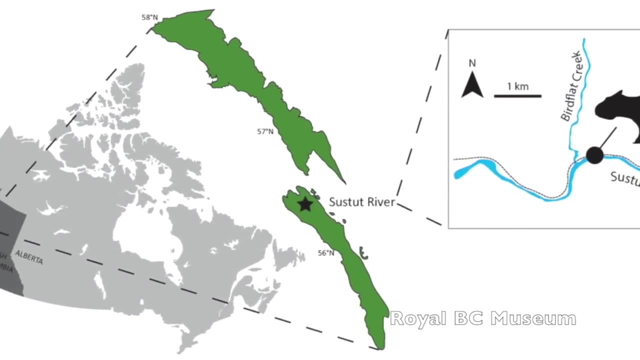 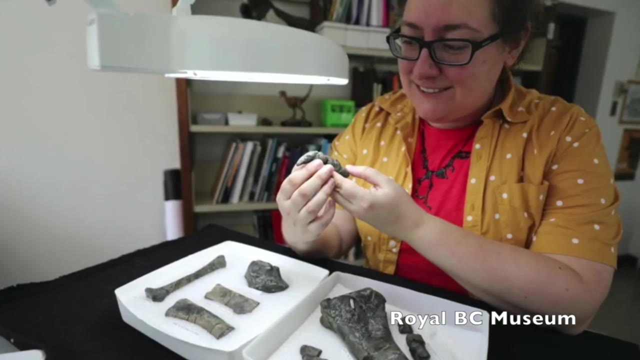 discovered quite by accident by geologist kenny f larson in 1971, who was exploring uranium and thorium deposits on a now abandoned rail line along the sustent river in british columbia, canada. it wasn't until dr victoria arbor, curator of paleontology at the royal british columbia museum. 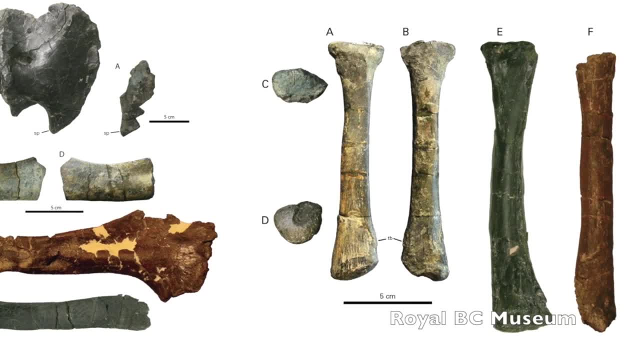 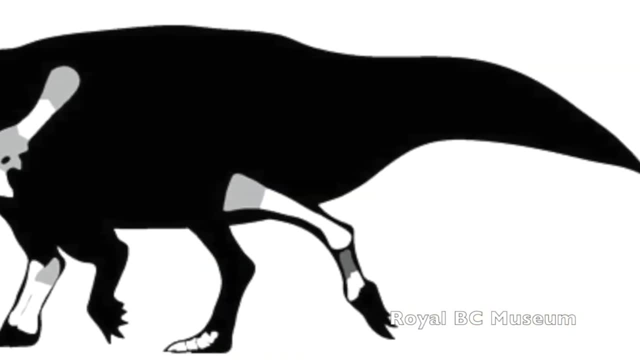 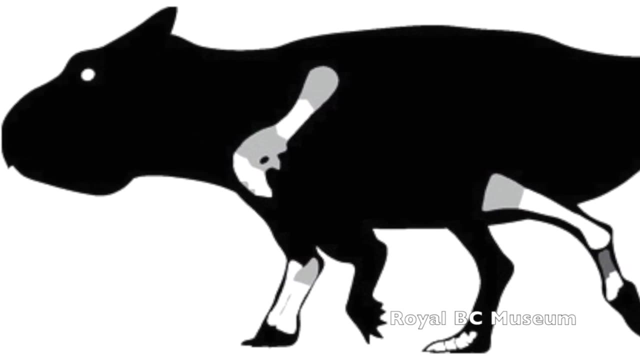 took a closer look at the fossil larson had discovered and found it to be an entirely new species. the scientific name pharasaurus sustenensis means iron lizard from the sustet river. as a nod to the railway where the specimen was discovered, the artwork i contributed for this discovery a fall day out. 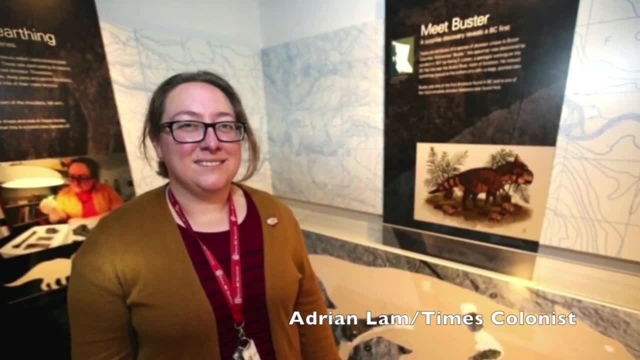 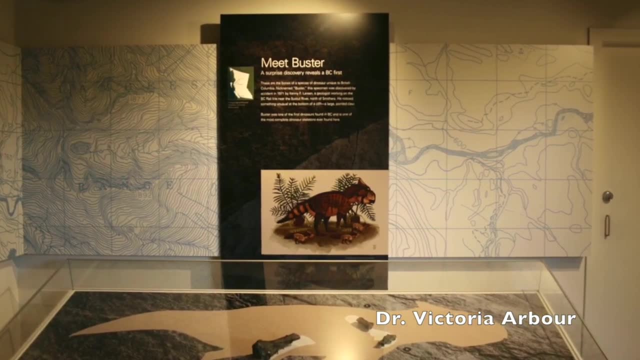 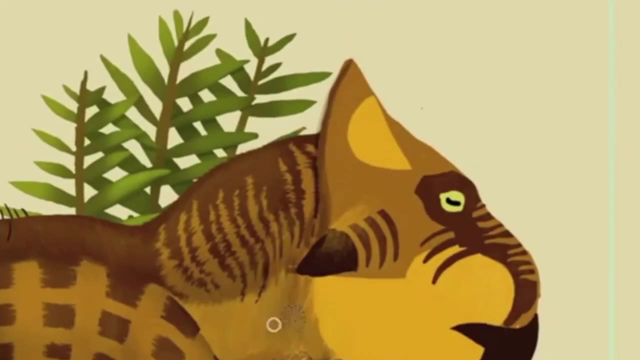 was featured alongside the fossil buster in the royal british columbia museum's pocket gallery for an extended exhibition lasting four months in the latter part of 2019 and early part of 2020. i originally painted a fall day out back in 2014 for a joint art show in anchorage, alaska, called shields and spears, with my husband. 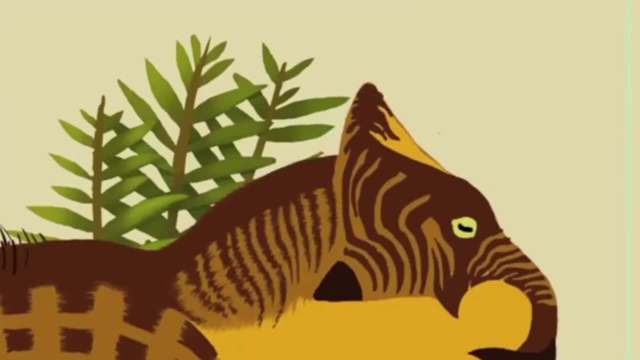 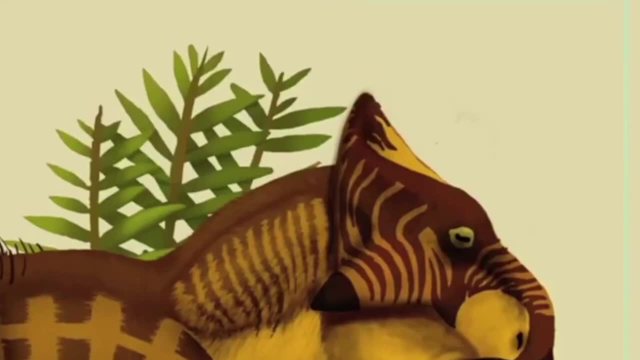 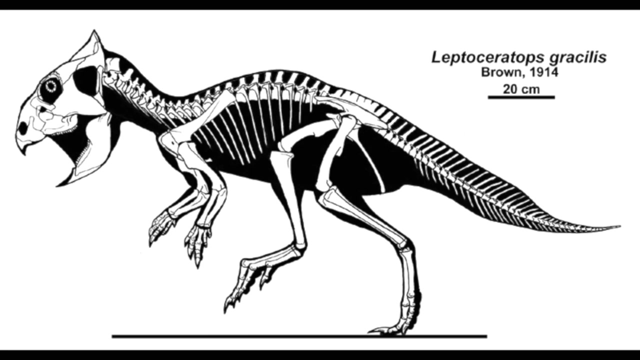 fellow paleo artist, scott elliard, and fellow paleo artist, researcher and friend zachary miller. i created this painting entirely in photoshop using a wacom cintiq art tablet and i used this great skeletal drawing by artist jamie hayden as the basis for my proportions. after all, a good 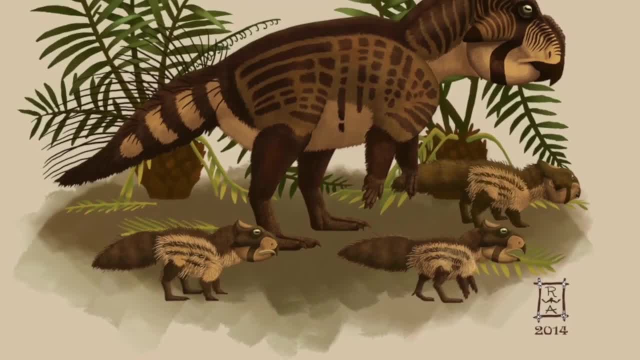 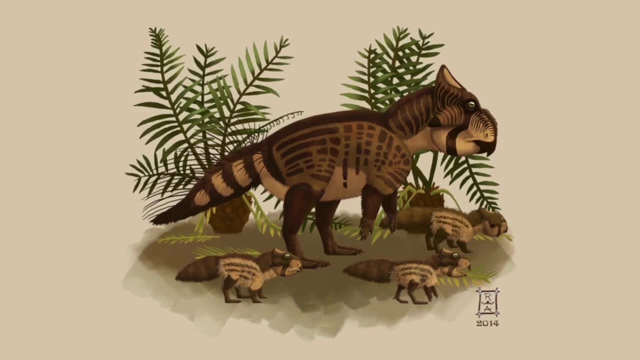 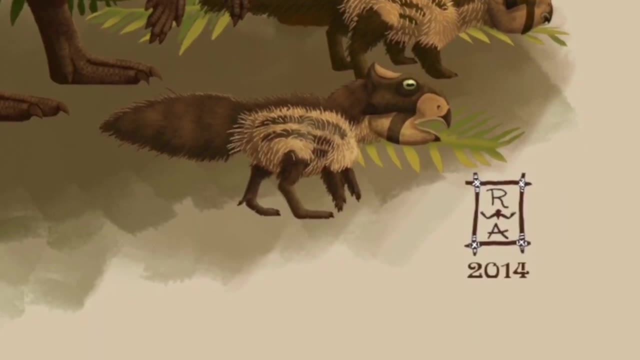 skeleton makes a good body. i included some ground hugging cycads for scale and for framing. i used a vignette with the ground colors to give it a storybook feel. this was also an attempt to expand my art and to do a more painterly approach than my normal line work style. if you like this painting of buster and would like 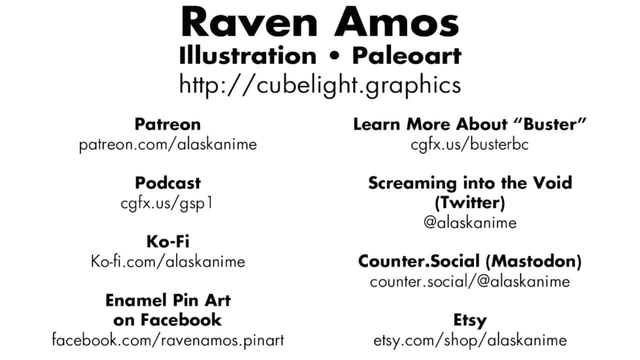 to see more of my art, please visit my portfolio site at cubelitegraphics, where i also have links to my patreon, my online apparel shops, my etsy store and my art store and my art gallery, and I'll see you next article again. you, where you can also catch episodes of my new podcast. 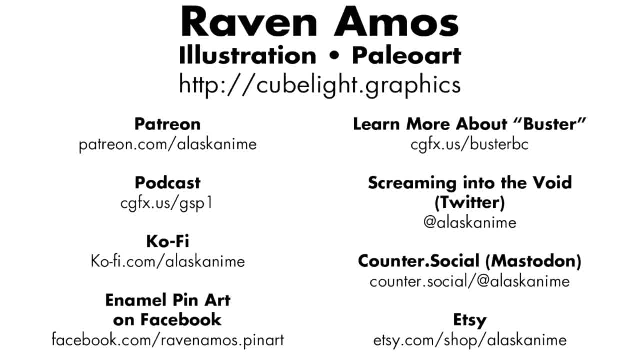 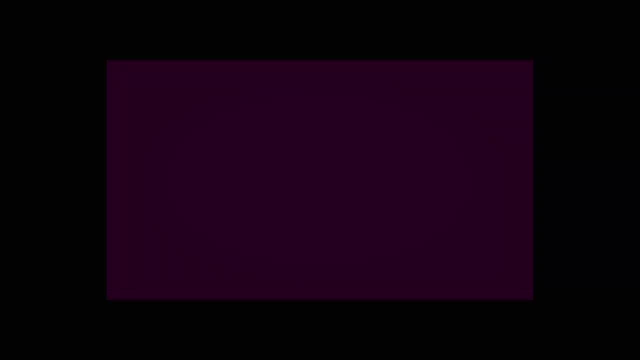 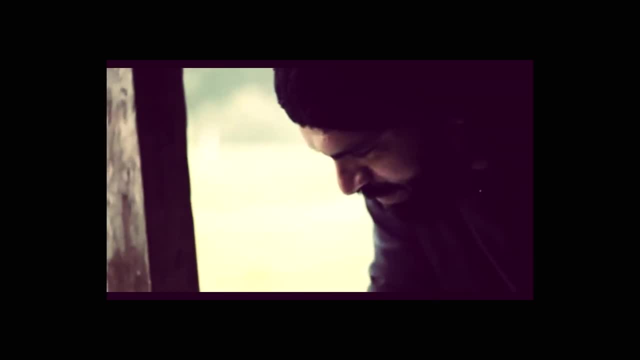 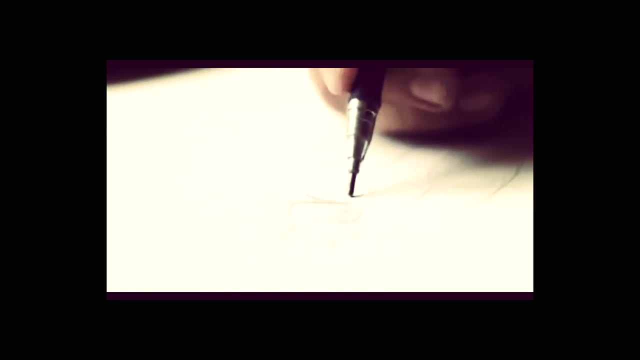 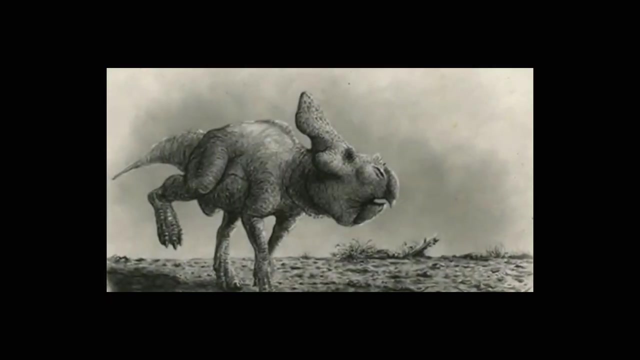 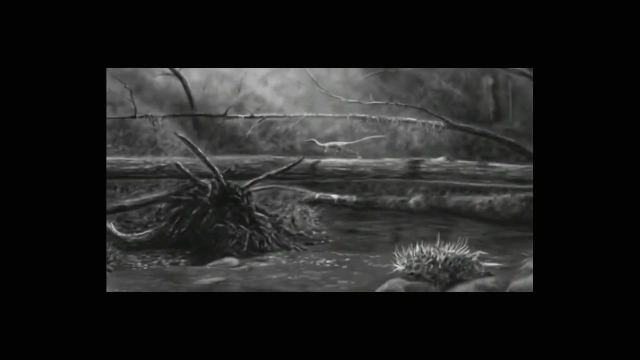 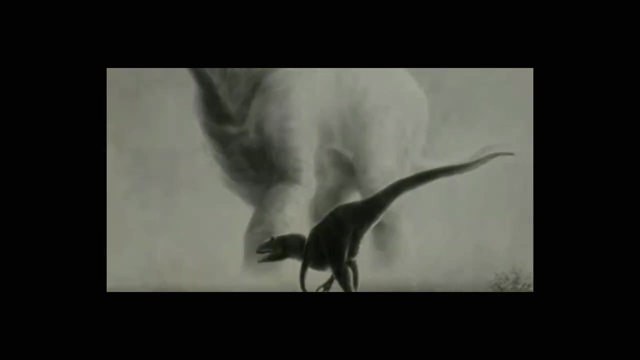 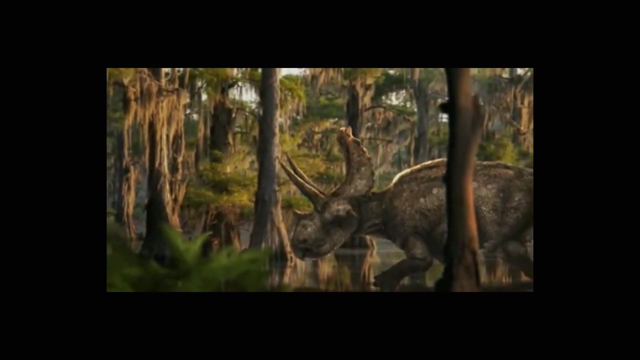 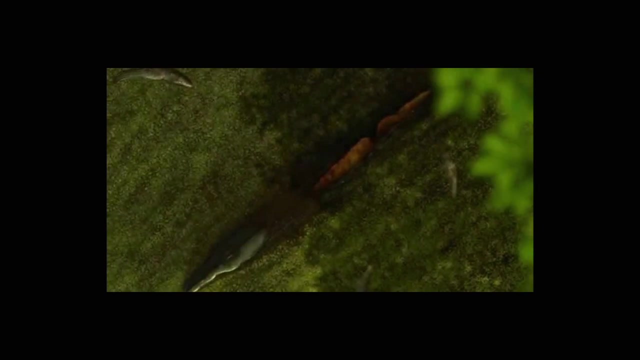 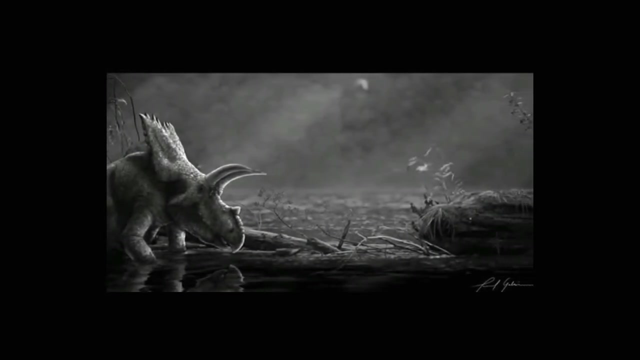 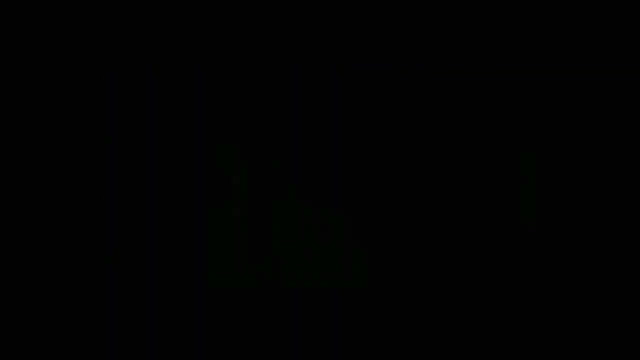 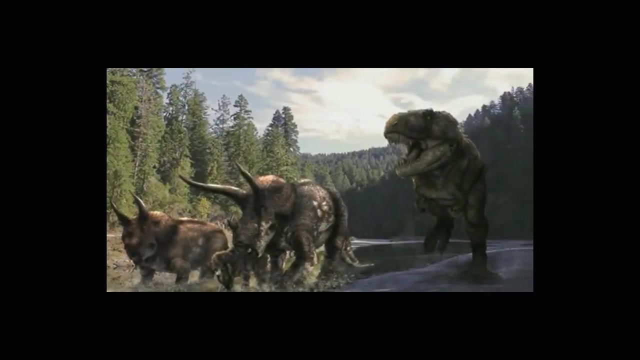 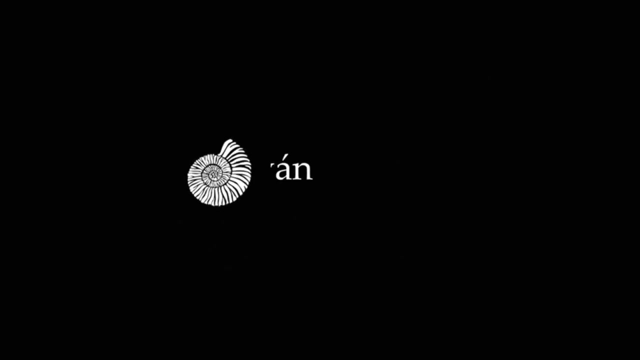 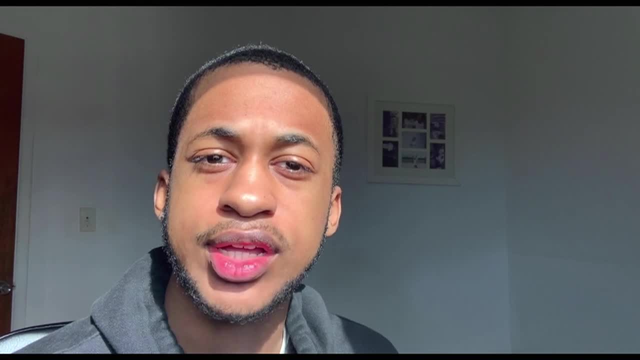 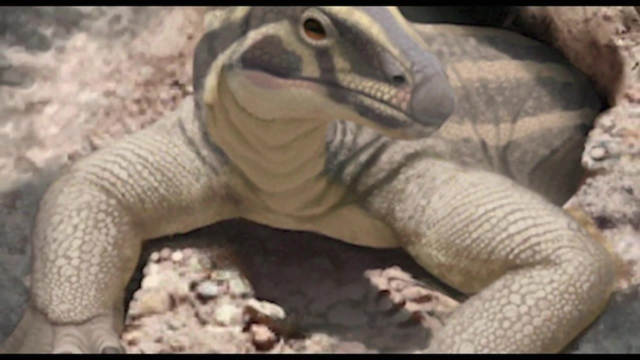 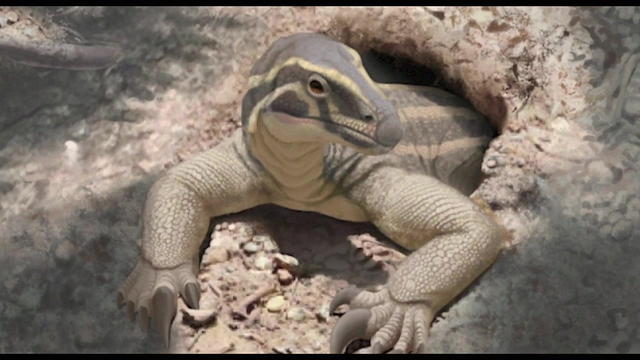 And this particular illustration that I have is of a drapanosaur called Skybalonix. Skybalonix is this small-sized drapanosaur that we have from the Blue Mesa, member of the Petrified Forest, And this guy has these really interesting claws to it. 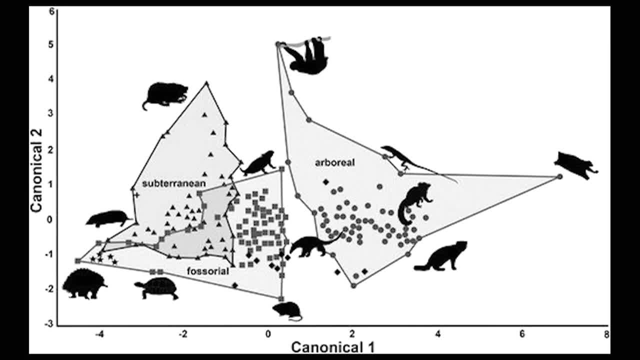 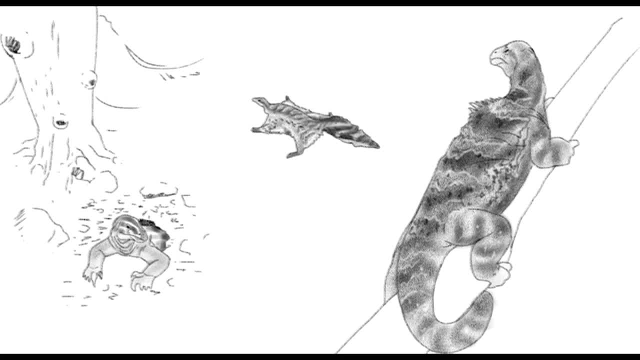 that really tell us a lot about its lifestyle. So, unlike other drapanosaurs, which have really long and thin claws that are really good for climbing trees, this guy has instead really short, blunt and massive claws that would have been great for digging. 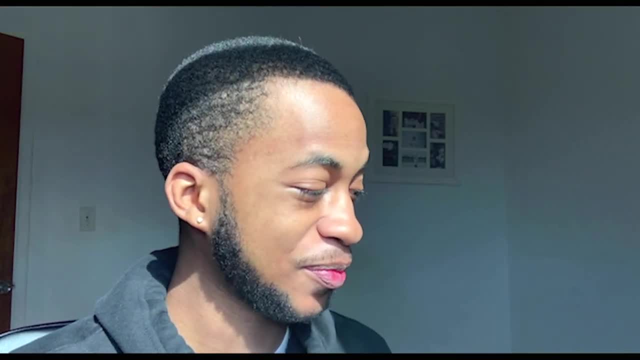 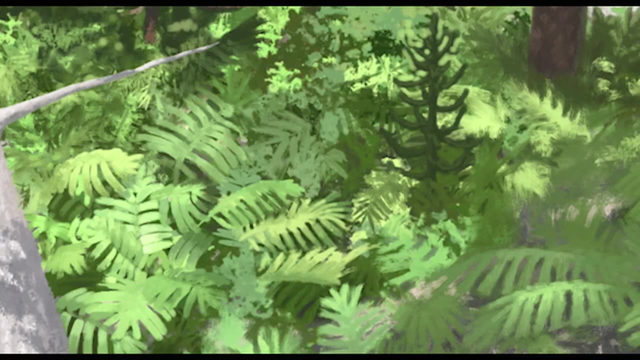 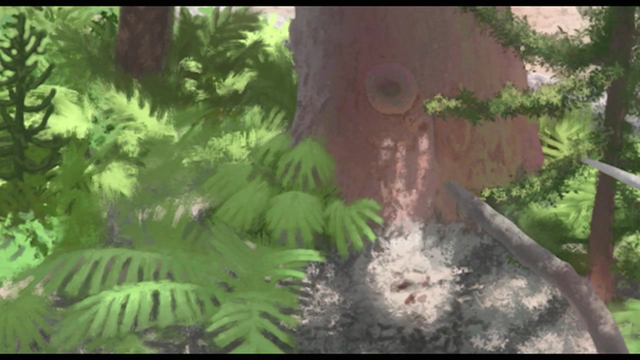 This illustration was a lot of fun to work on, Literally, and a little sarcastically- Mainly sarcastically- in the sense of having to paint the flora. The plants were definitely not easy to paint, but it's definitely satisfying to do the proper research. 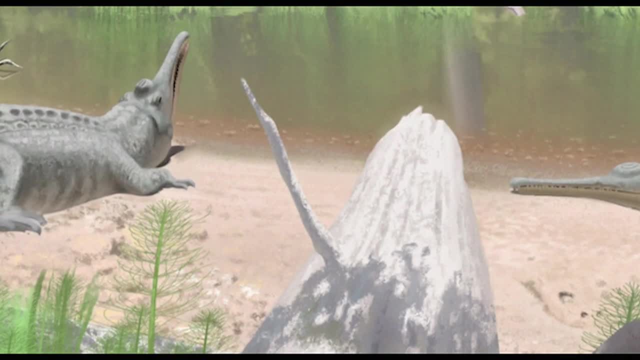 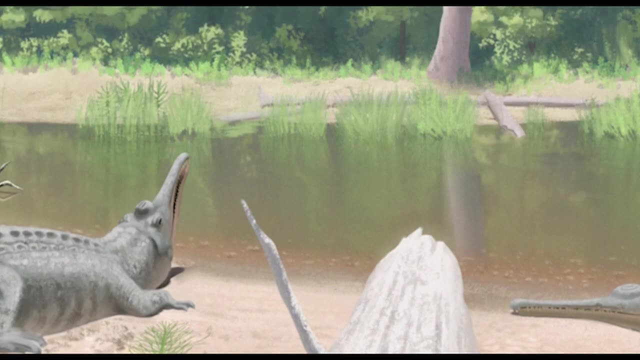 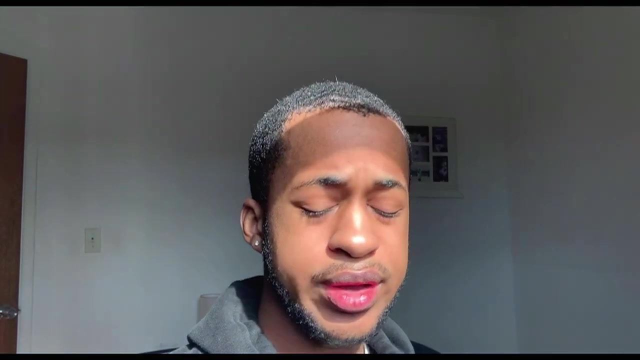 into the type of flora that would have been present in the environment, so that then you can properly give it due justice and bring it truly back to life and help support the key animal that is being showcased in the piece. Now, a lot of this illustration was started off. 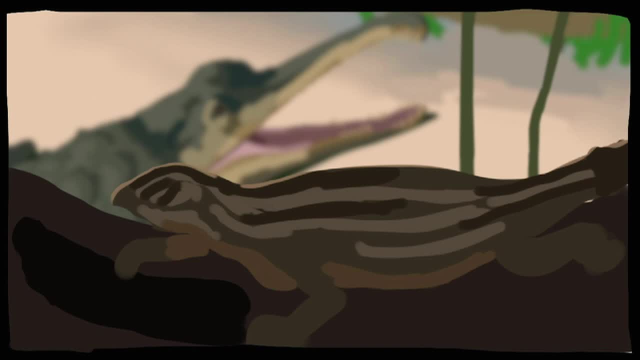 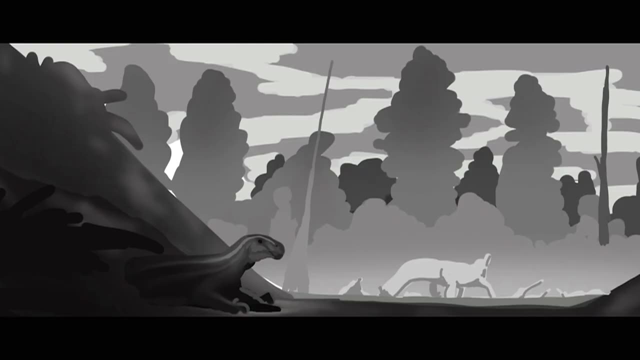 with me first trying to block out how I wanted to approach it from a composition standpoint. I went through a few different options, but I eventually landed on one which I typically go for when I'm usually doing a lot of my paleo art pieces. 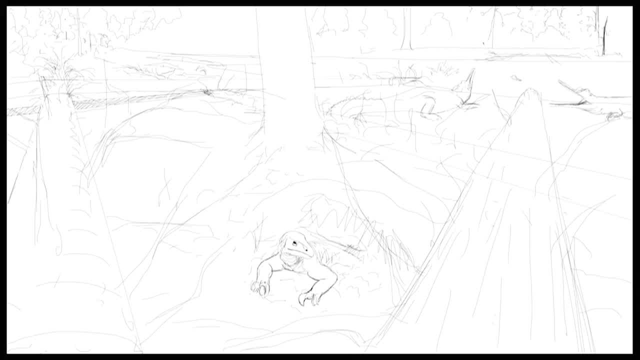 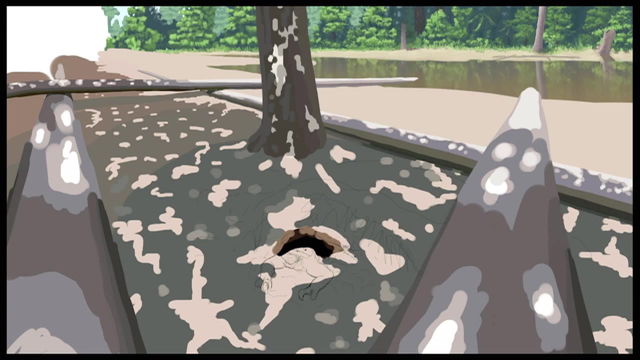 which is almost as though I'm a photographer in the actual scene, And I believe photography definitely communicates the presence of an animal or an environment better than maybe some other approaches to composition. So I went for that, almost like a fish eye lens approach to it. 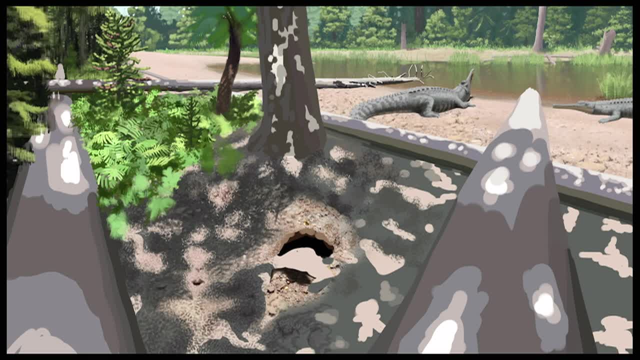 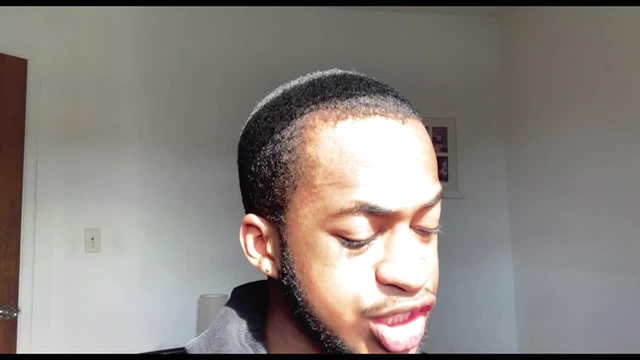 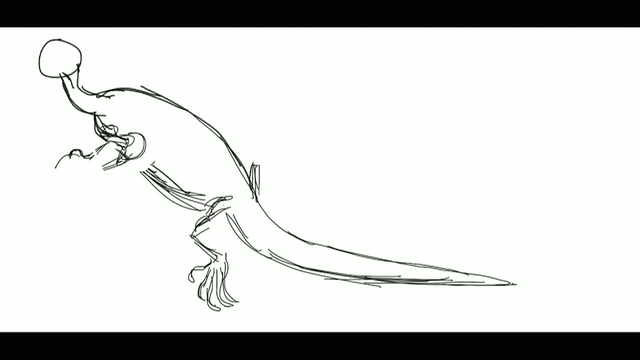 That way you could get the main character and then everything else in the background without having to really sacrifice much space. Once I was done with all that, I could move on to actually getting to the main character, And even before that, designing this actual guy was a little tricky. 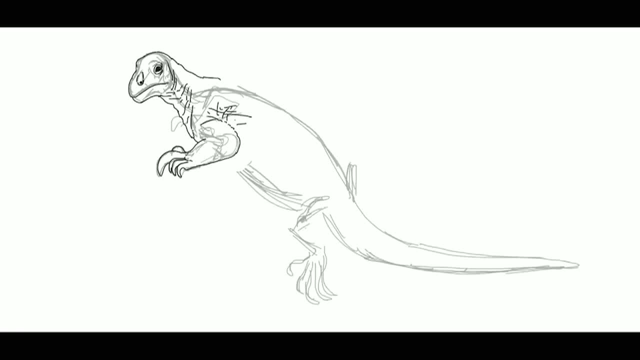 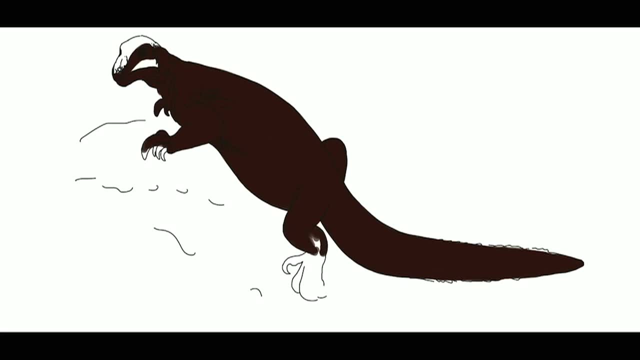 but fun at the same time, because I was more or less creating a speculative animal that we don't really have any tangible fossils for other than its claws, So I was mostly relegated to looking at modern digging lizards and other small burrowing tetrapods. 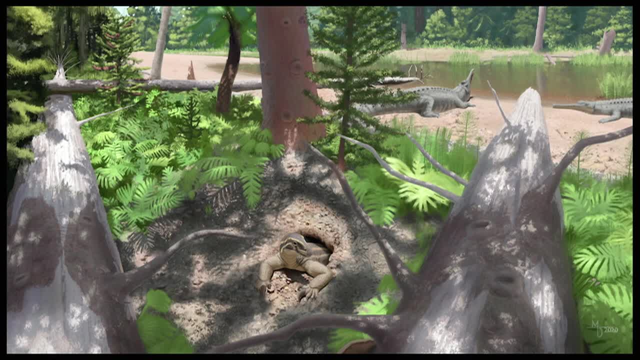 that really have this kind of lifestyle, while still taking into account the weird and bizarre anatomy of Grypanosaurs, especially with their weirdly tall backs and weird arm and shoulder morphology. And that's that If you're interested in seeing more paleo art. 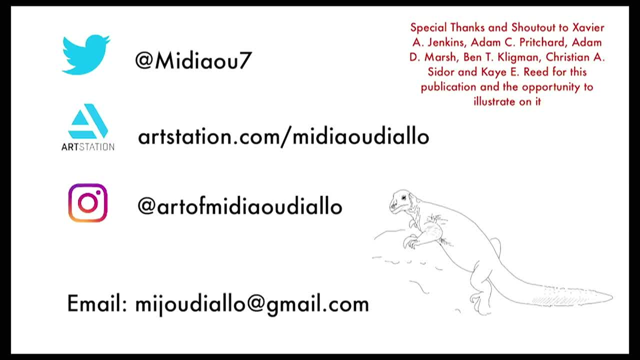 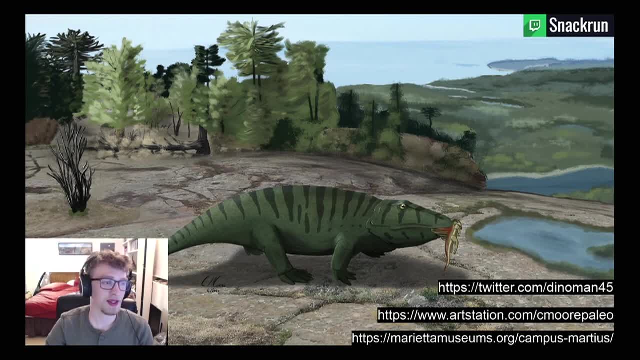 definitely follow me at these sites. We'll definitely see some more coming soon. My name is Connor Moore and I'm an aspiring paleontologist and paleo artist. I live in Indiana. I'm currently trying to apply for PhD graduate schools for next year. 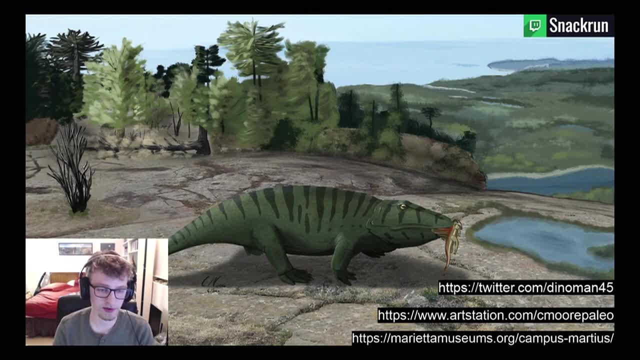 But in the meantime I've had a wonderful opportunity to work as a guest curator at a small museum in Marietta, Ohio, called Campus Marshes Museum. I posted the link here at the bottom so you could go check it out if you'd like. 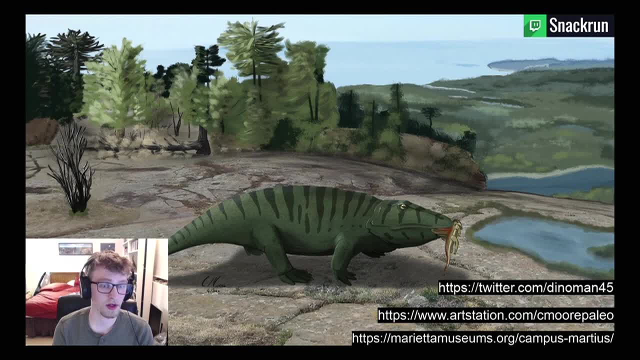 We're focused on early Permian local fossils that have been found there, Just kind of forgot about for the last six years or so years. So part of my job has been to really showcase you know what's going on in the environment. 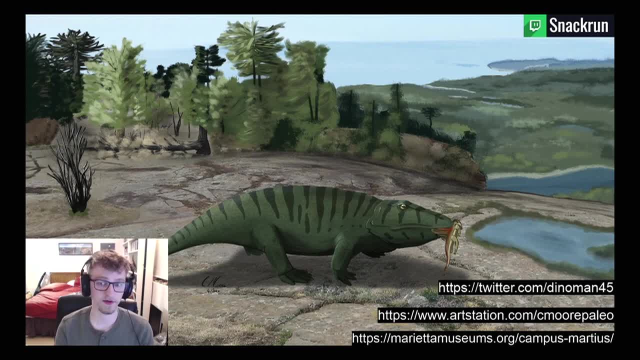 and what's happening in the environment and what's happening in the environment and what's happening in the environment, And I get to showcase and present these fossils in a really fun and exciting way. And I get to design all the walls and choose the paleo art for the fossil reconstructions. 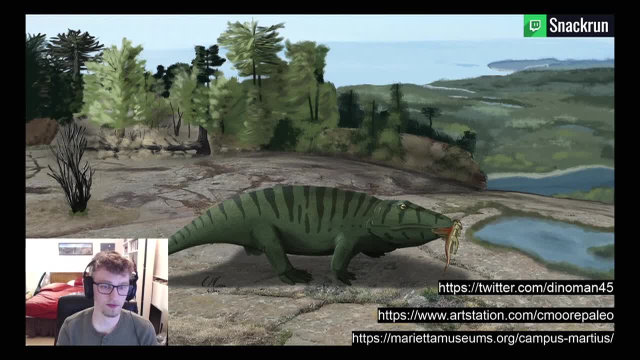 But unfortunately, being a kind of really small museum, we didn't have enough funds to really support a professional paleo artist. But luckily I've had sort of a general art background and I've always wanted to do paleo art And I used to do, you know, a lot of paleo art, you know. 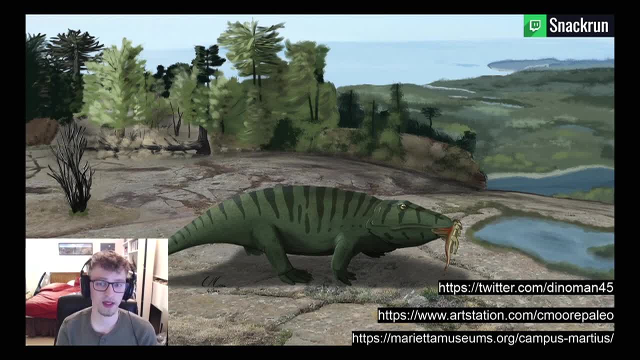 and I've always wanted to do paleo art and I've always wanted to do paleo art pencil drawings. but this really tested me in Photoshop- pencil drawings- but this really tested me in Photoshop- My Photoshop skills. I've definitely seen an improvement. 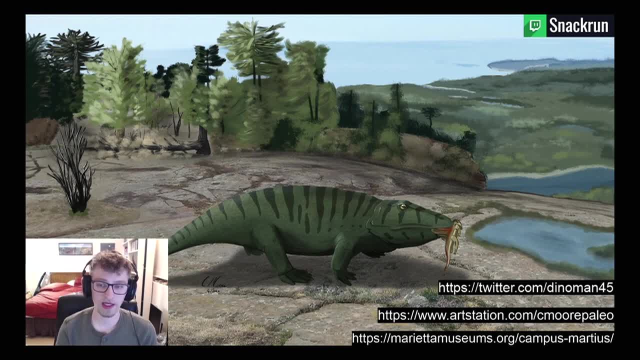 over the last year or so that I've been doing this And I just wanted to showcase two of my pieces of art here. You could go check out the rest at my art station at Seymour, Paleo, And you can check out my Twitter: dynoman45.. 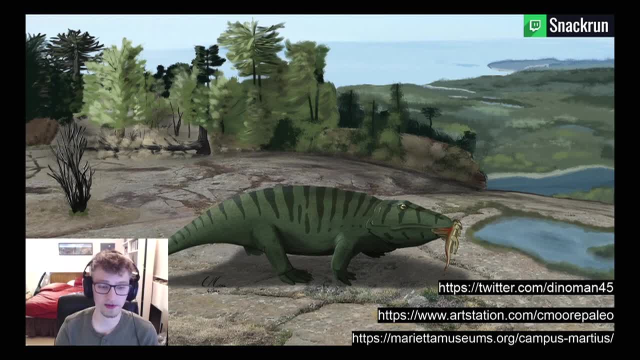 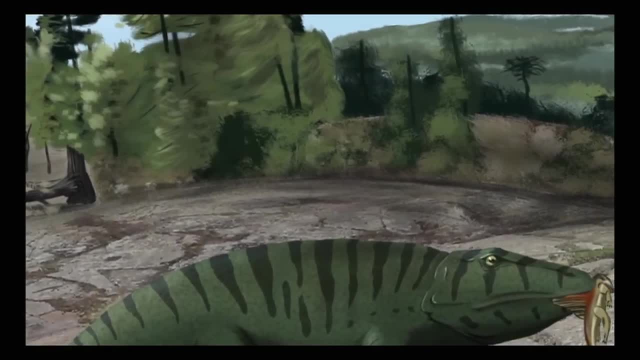 And I also do stream on Twitter And Twitch. sometimes you can find me at twitchtv: slash snackrun. The one that I have here is a Areops. It's about a three meter long carnivorous terrestrial amphibian that lived during the Carboniferous. 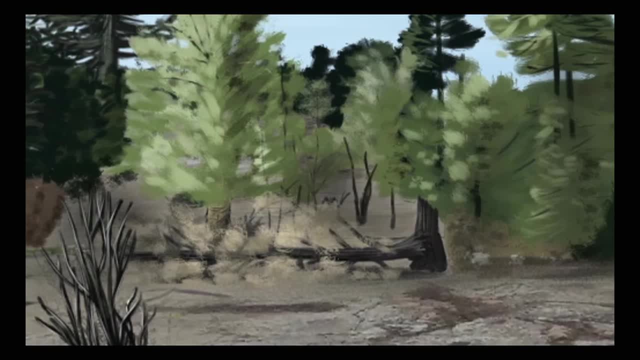 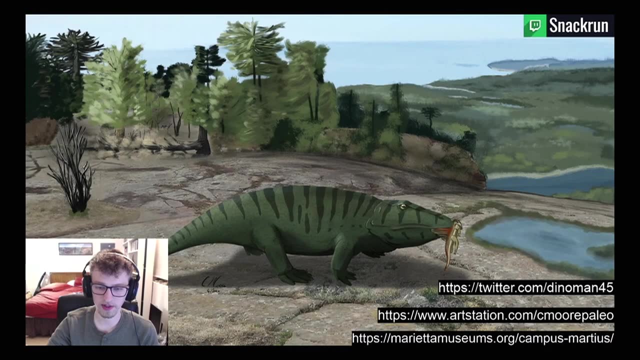 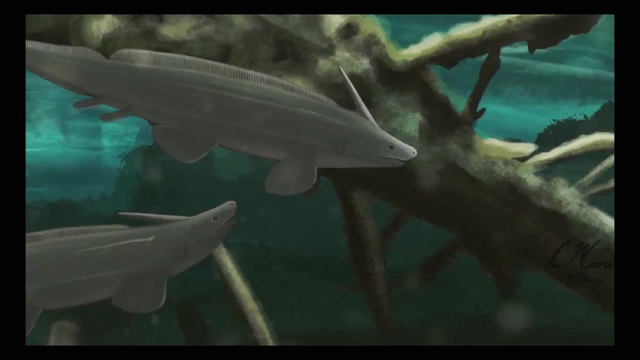 and early Permian. This was really challenging and really fun to do. Trees are really hard, but it was a lot of fun to learn how to do that. Second one that I have here to show is a two freshwater Xenocanthus sharks. 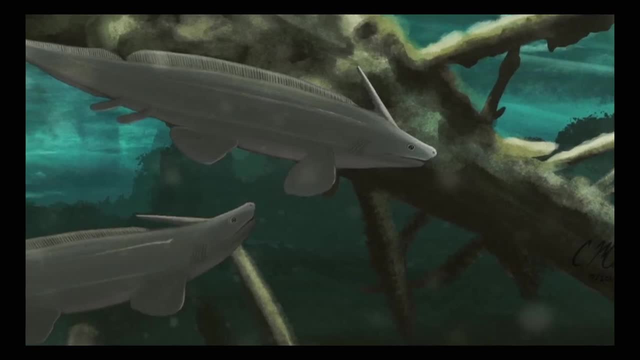 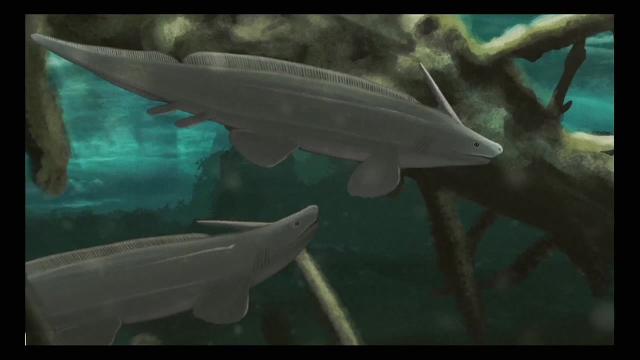 Also lived during the early Permian And I'd never done an underwater scene before, so this was very hard, but I love how it turned out And I hope to keep improving. So if you would like to talk to me more about dinosaurs, 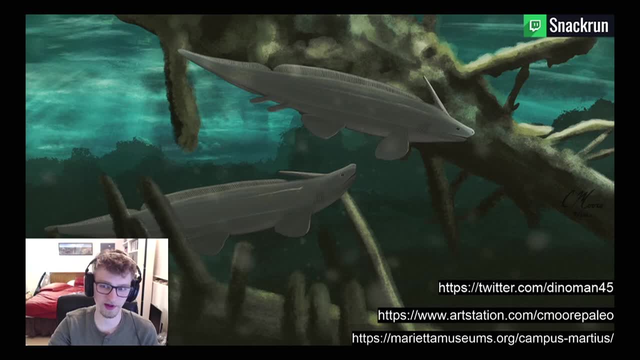 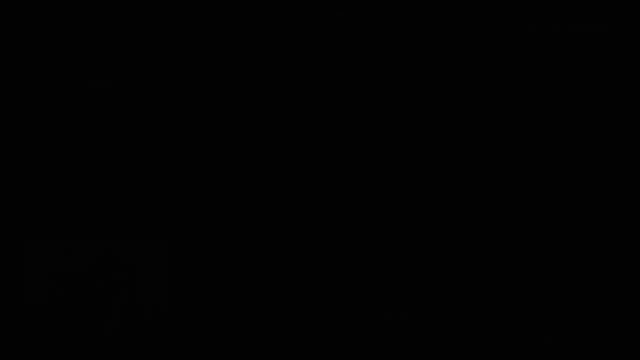 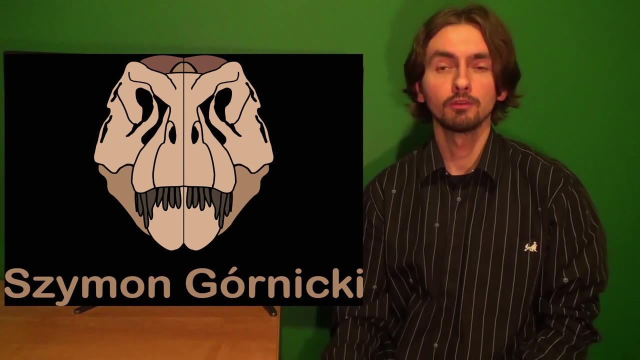 or the early Permian or whatever else paleontology related. just reach out to me. I can be a founding newer. Thanks for checking me out. Peace, Hello everyone. How are you doing? I am Szymon Górnicki, paleoartist and paleontologist. 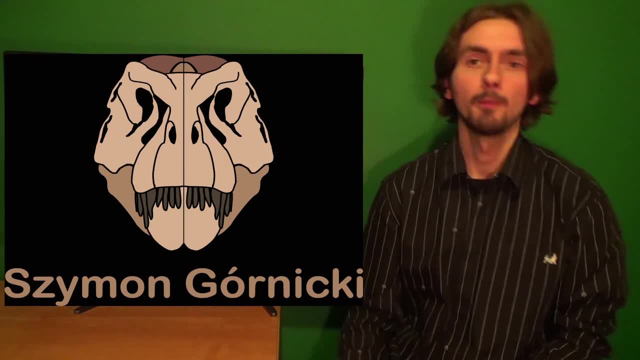 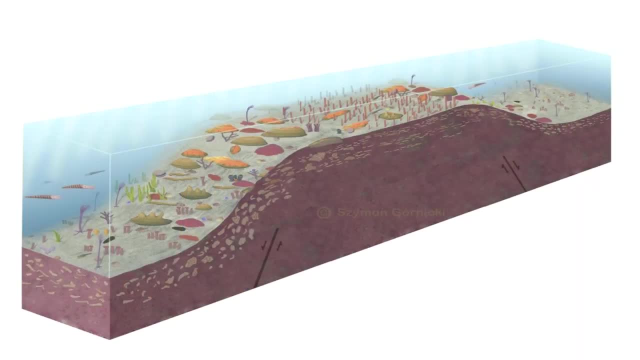 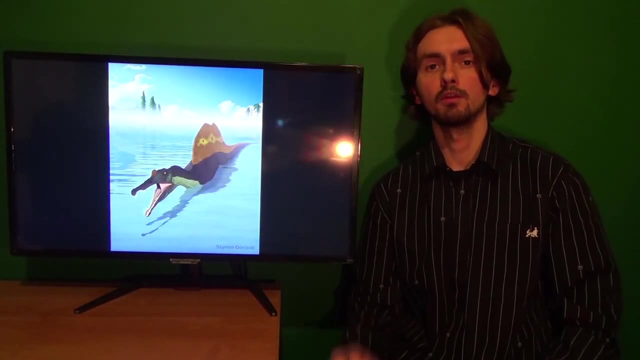 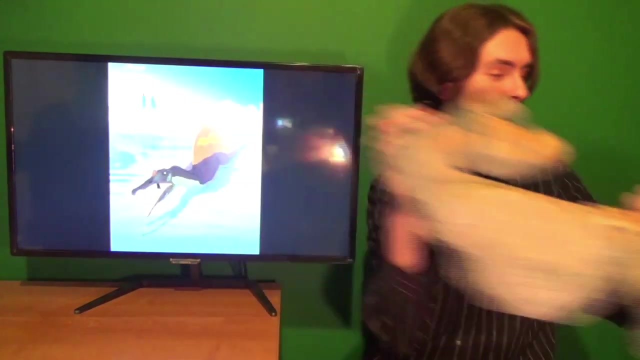 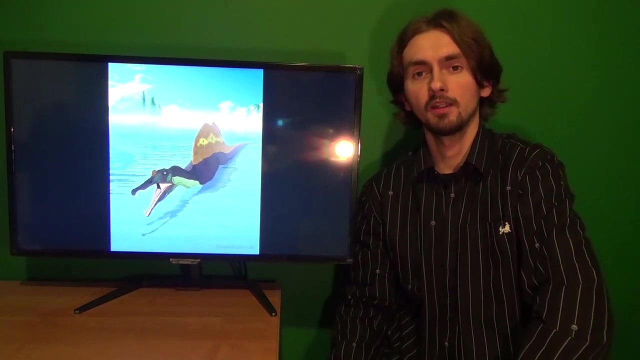 from Poland. Mostly I do digital 2D paleo art, So some examples here. I also made traditional 3D models. This is a picture of my friend, his little friend. I write articles focusing on paleoart and Polish Triassic. 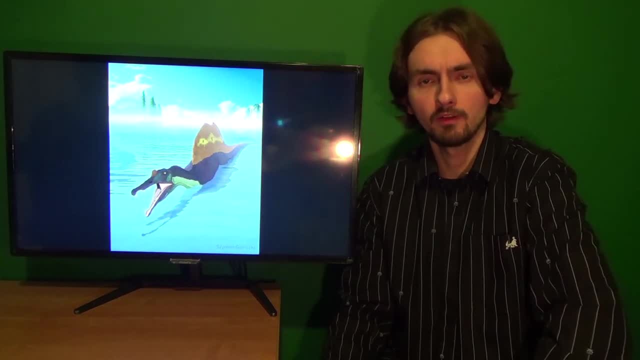 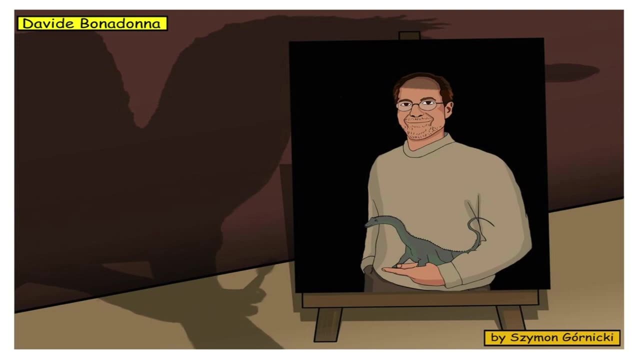 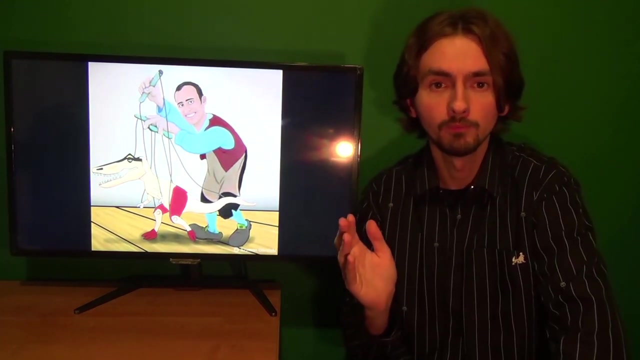 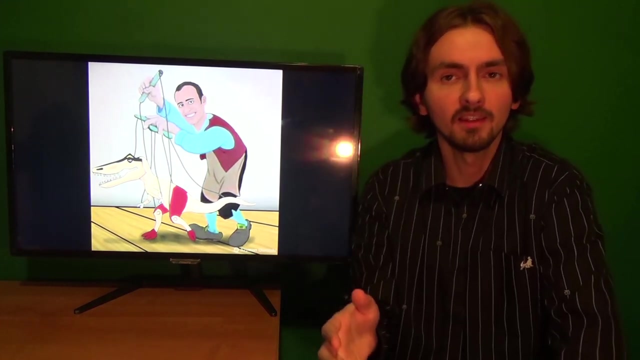 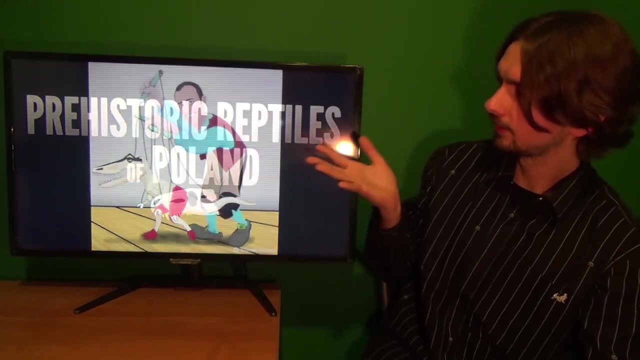 Distinctive part of my creative work are humorous graphics like this, But the most important is what I am doing now. I am using my computer Now Together with my right hand, Joanna and other talented, wonderful people from different passions, I am making prehistoric reptiles of Poland. 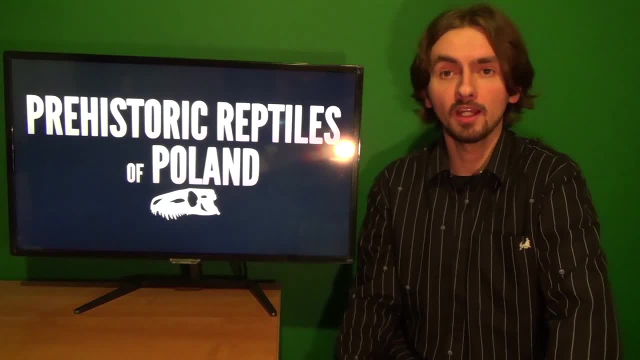 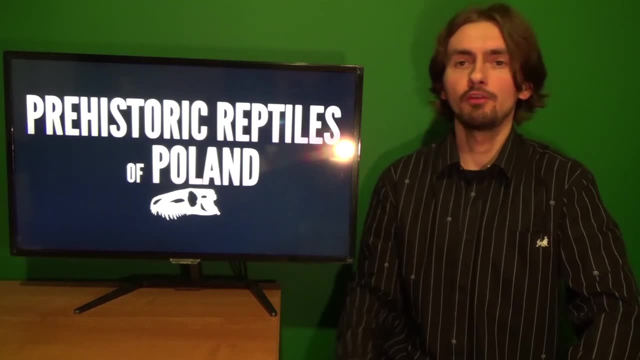 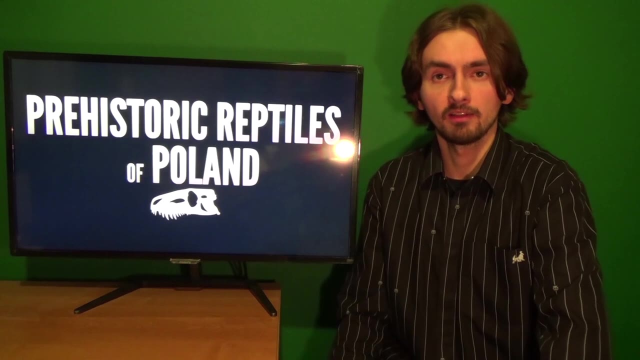 This will be the first independent CGI animated paleontological documentary. This will be the first independent CGI animated paleontological documentary. This is my first video. This is my first video. This is my first video. create a film in walking with dinosaurs style. in this movie, science will be the most important. 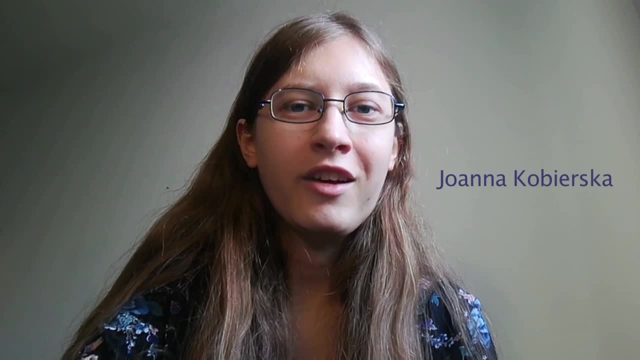 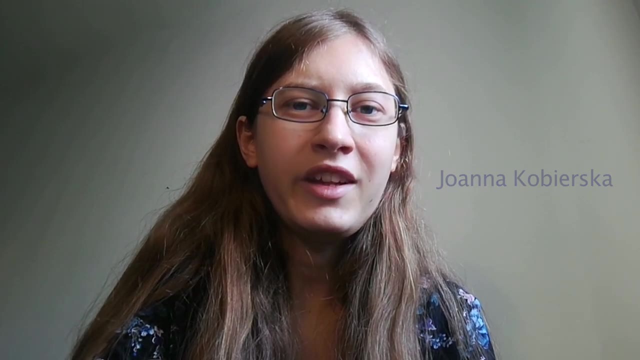 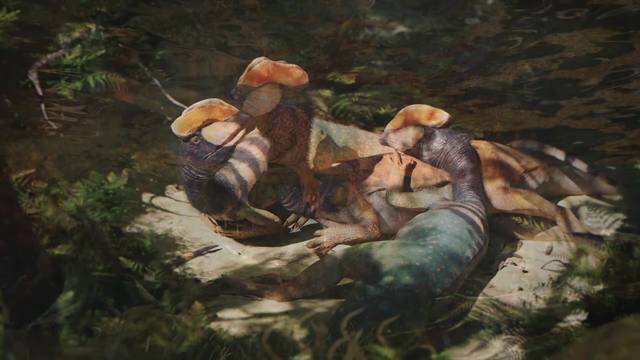 thing. Hello. I'm Joanna Kobielska and I'm a 3D artist most interested in reconstructing prehistoric fauna in 3D art mediums. I try to show my subjects in most lifelike way possible where live photography and observation. 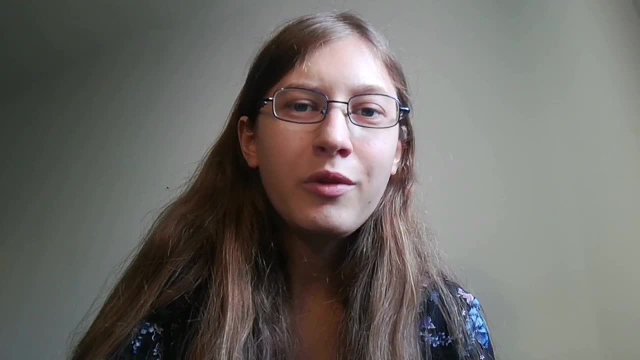 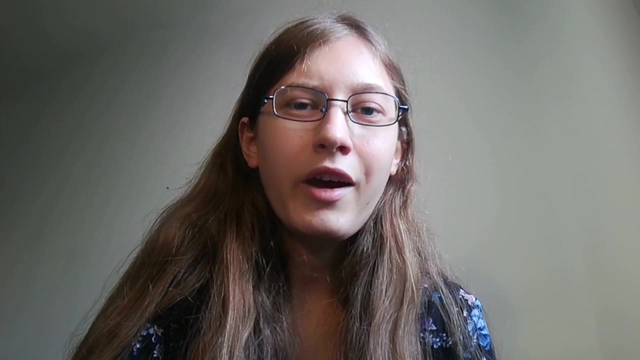 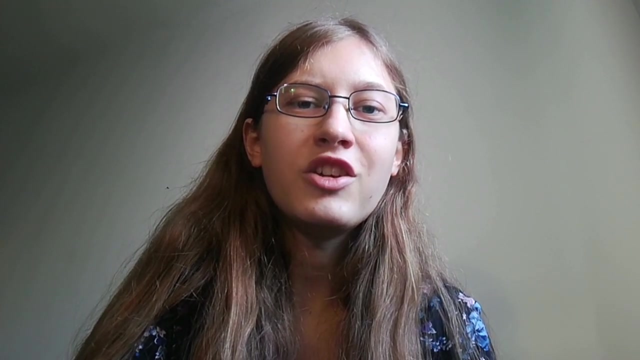 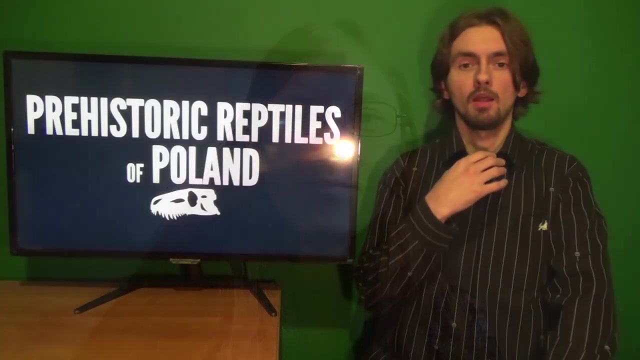 of extant animals are my biggest inspirations. Together with Szymon, we are trying to bring to life rather obscure biota of Jurassic Poland. We are combining newest discoveries with cutting-edge CGI to get most realistic representations of those animals. So our project is made by paleoentusiasts for paleoentusiasts. 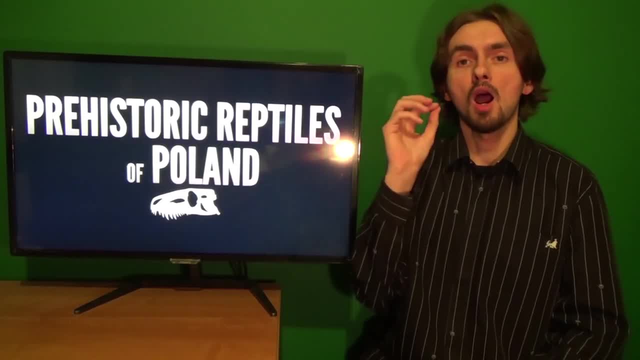 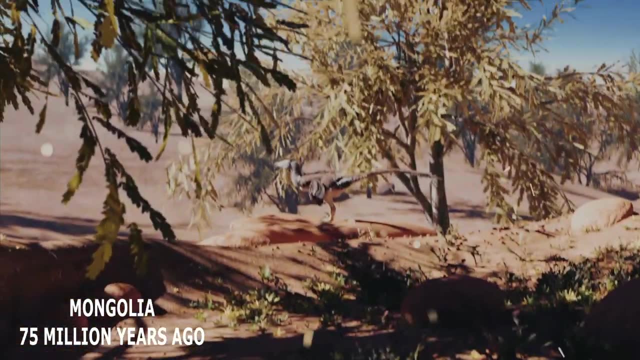 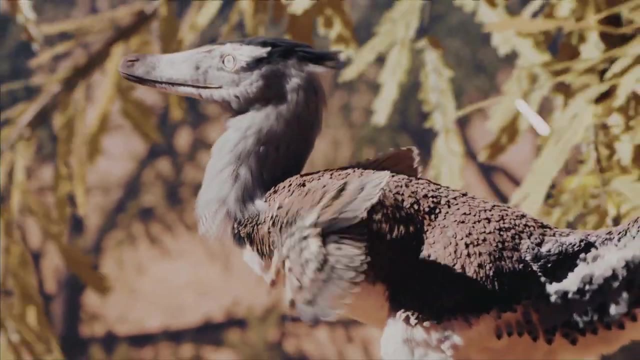 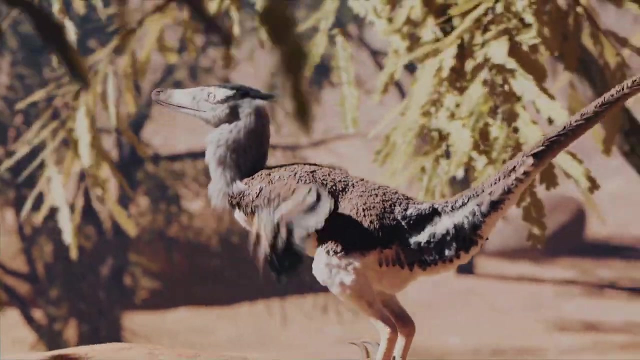 Thank you for your time and now our demo. See you, Let's see what we can do. Born of the prehistoric Gobi desert. amidst the dunes, a male velociraptor prepares for his mating dance. He intends to catch a female's attention. 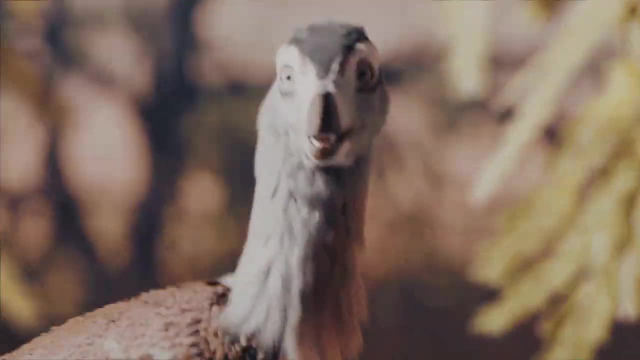 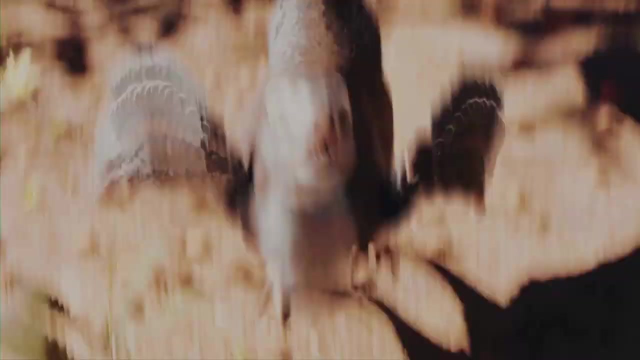 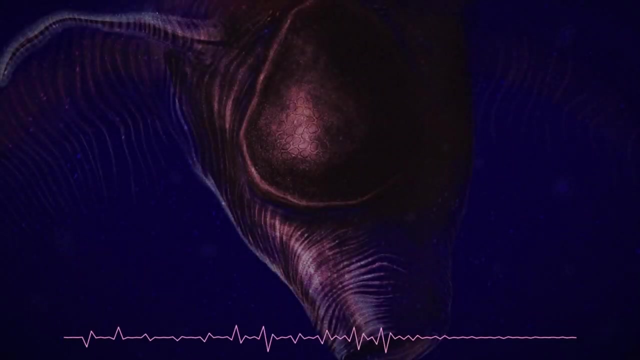 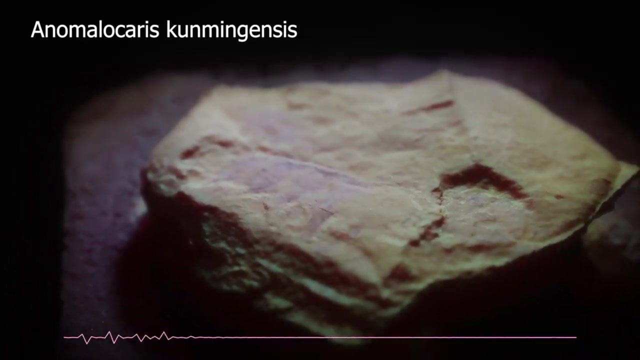 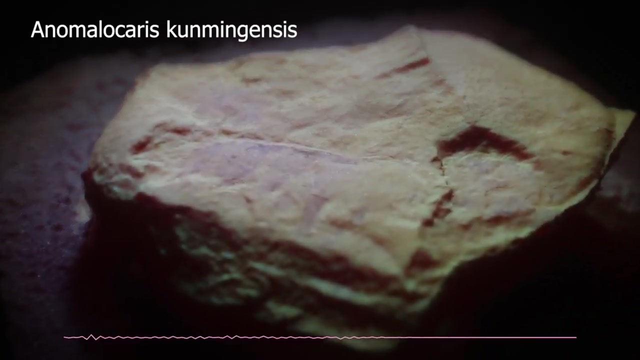 Unfortunately, our cameraman has disturbed his territory. Hi, I'm Prehistorica. I am an invertebrate-centric paleoartist with a specific interest in a group of animals called lobopods and radiodonts. General rule of thumb: if it's one of the famous Cambrian weirdos, it's probably a lobopod. 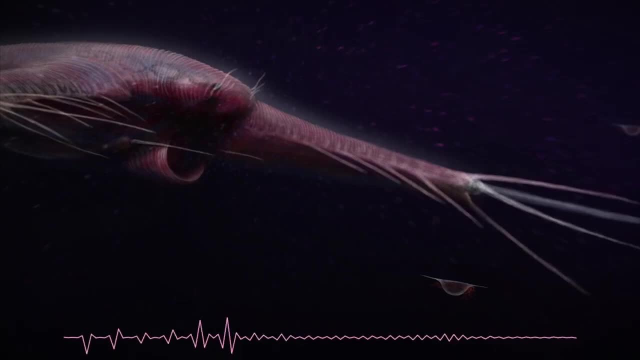 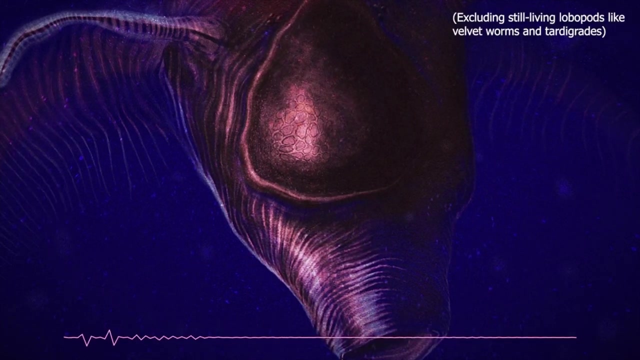 or a radiodont, Think animals like Aishaia Hallucigenia, I don't know. All of them are lobopods and radiodonts And if my records are correct, I have drawn at least half of every lobopod species known. 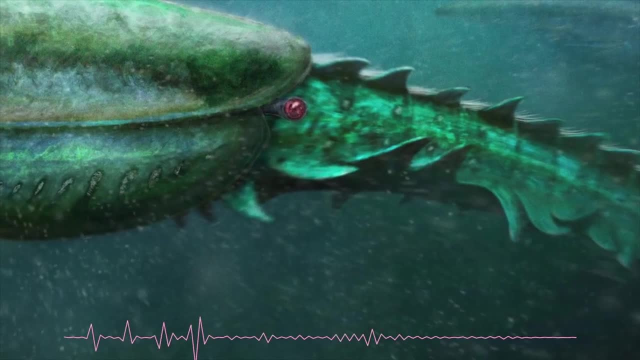 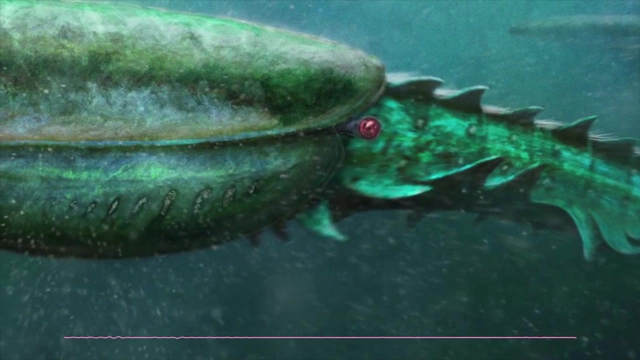 to science, But this- this is the first one that I was ever commissioned to draw. This is Ajiracossus benmulai. It is a giant herded radiodont that came after the Cambrian. It's the first one I've ever drawn. 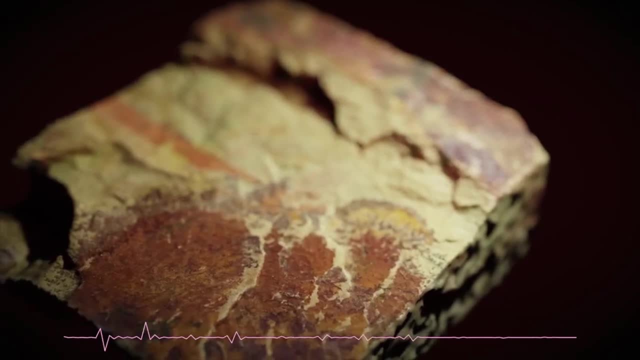 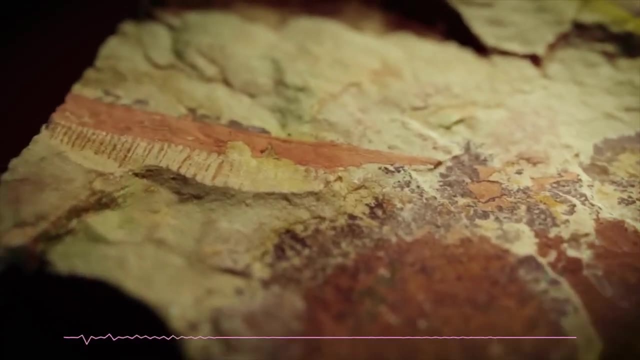 The first named radiodont to be discovered in the Ordovician and it comes from the relatively cold polar seas of Fezawatta. At the end of the Cambrian and at the beginning of the Ordovician there was a huge evolutionary 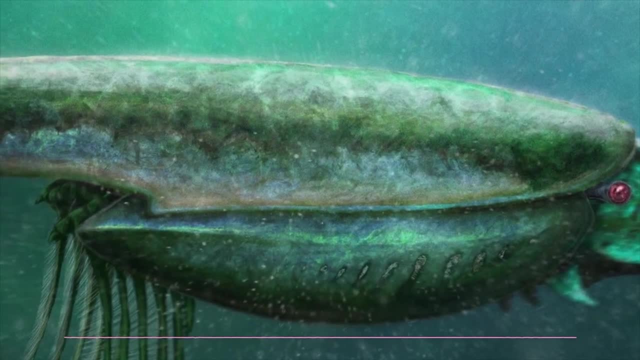 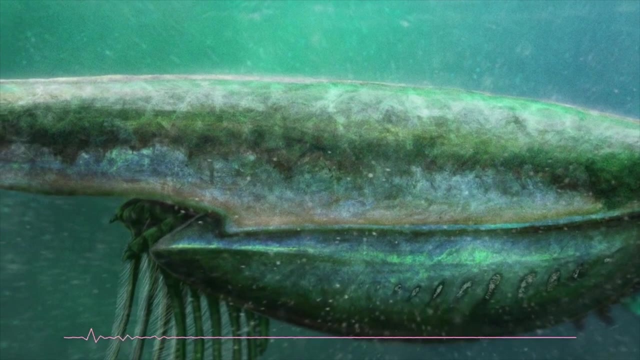 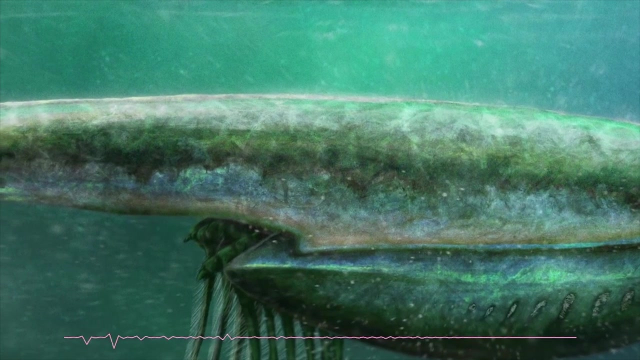 radiation event called the Great Ordovician Biodiversification Event, or for short GOBE, And among its many effects it marked a significant increase in the populations and diversity of plankton And in turn also increased the diversity of animals that feed on the plankton. 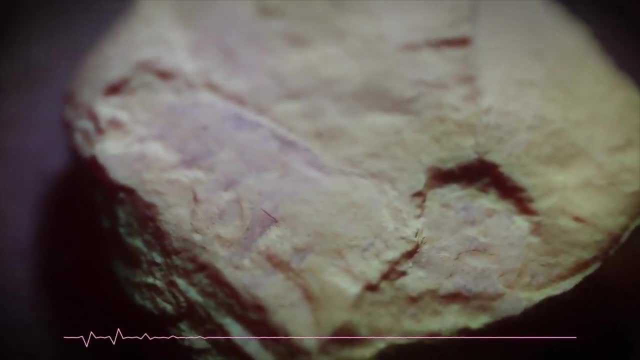 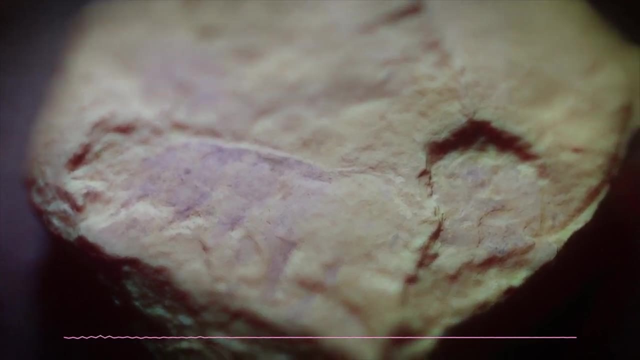 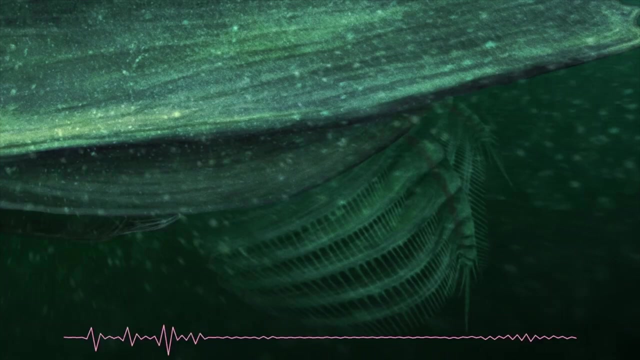 This includes Ajiracossus. Prior to this event in the Cambrian herded, radiodonts did not have a very diverse set of strategies for feeding. They almost always used their frontal appendages as a kind of filter basket. They would live close to the bottom of the sea and sift around in the mud and silt looking. 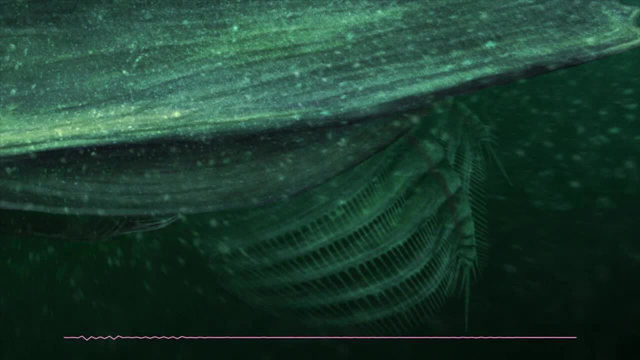 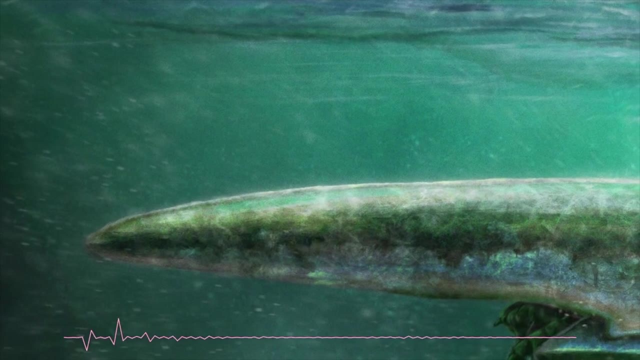 for small animals to feed on, Things like worms or hyalites, Maybe even trilobites, But as soon as the Fezawatta rolled around, herdeds went crazy with feeding strategies, And the first one that we know about is Ajiracossus. 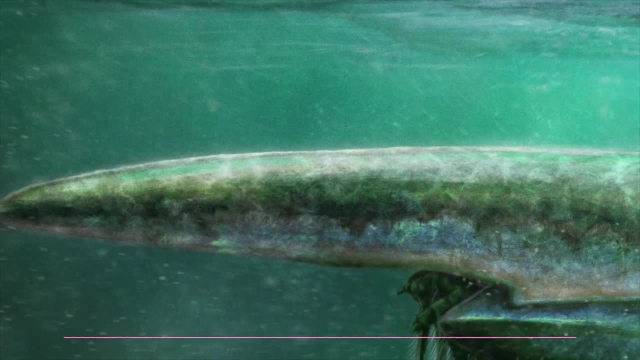 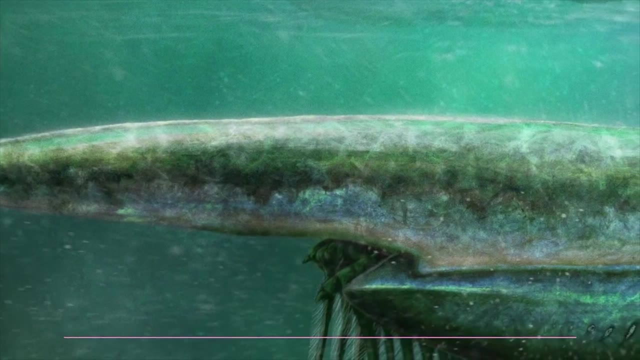 Running down the length of its relatively straight endites. the little spines that come down from the appendages were tiny but relatively long branching hairs that we call setae, And these hairs, in their great numbers, would have functioned almost exactly the same way. 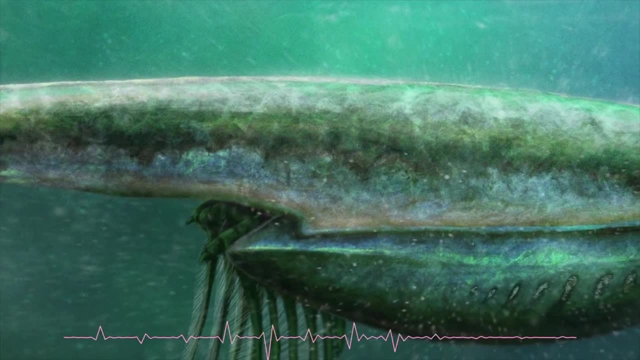 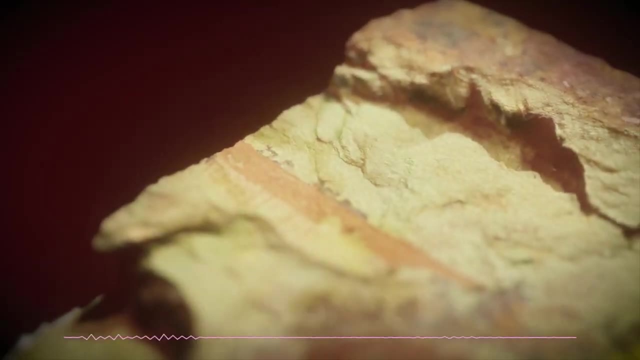 as baleen does in modern whales, Its great size would have drifted almost aimlessly through the sea, possibly in shoals, picking up plankton as it went along And after it collected a certain amount, or maybe after a certain amount of time has passed. 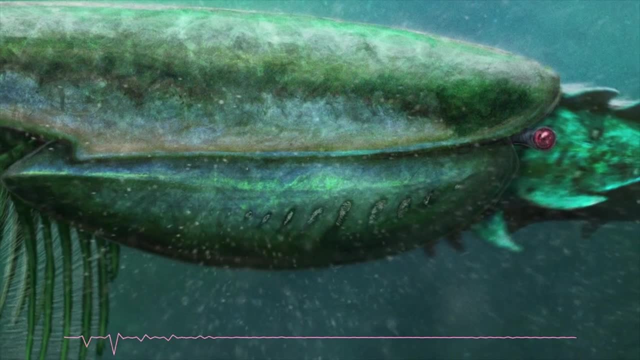 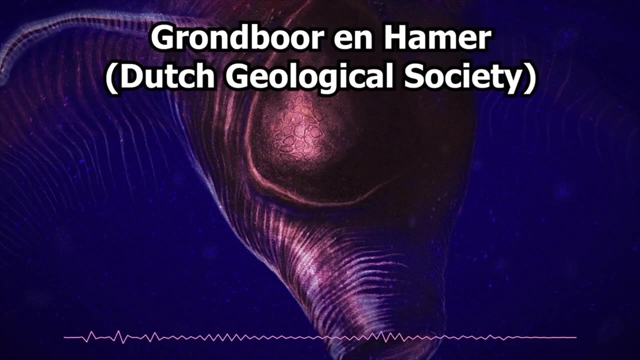 it would pass all the food into the mouth. All of this to feed an animal longer than an average queen-sized mattress. This work was paid for and done on the behalf of Grondboer en Hamer, a Dutch geological magazine, in which you will eventually be able to read more about Ajiracossus in the coming weeks. 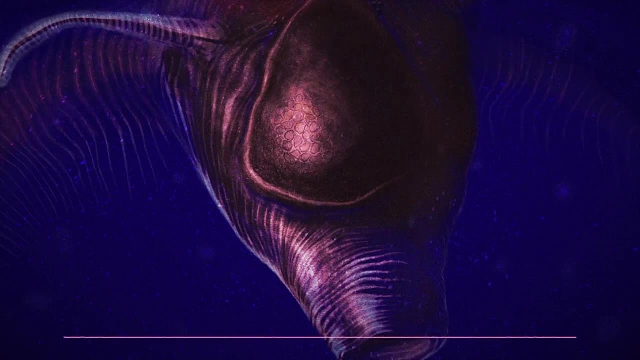 This work was paid for and done on behalf of Grondboer en Hamer, a Dutch geological magazine, in which you will eventually be able to read more about Ajiracossus in the coming weeks. I actually livestreamed a large portion of the drawing process for this piece, and it 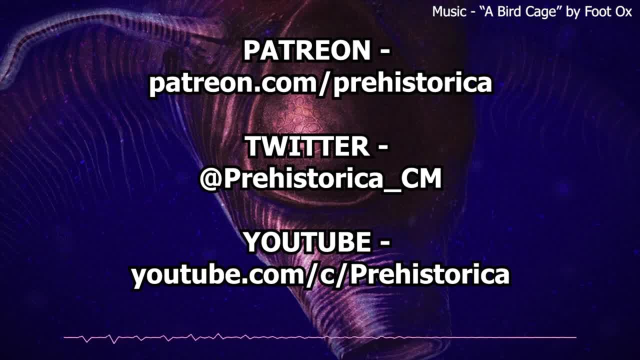 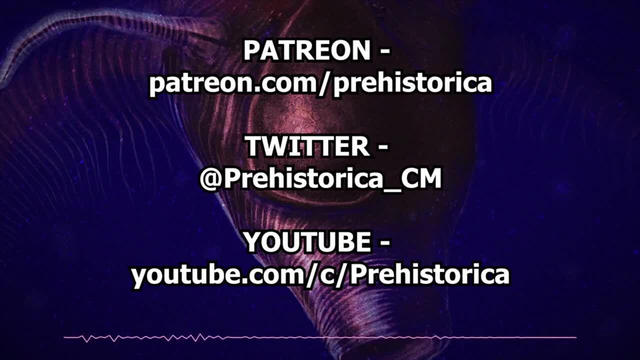 was a really good learning experience and I hoped that with the livestream I was also able to help out some people that wanted to see how I drew things, And I think that's about all the time I have to talk about worms and legs for now. so my